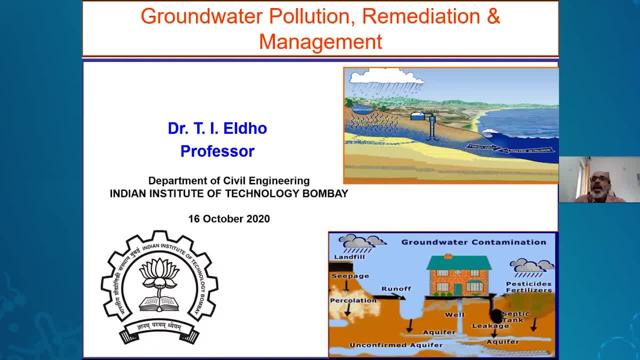 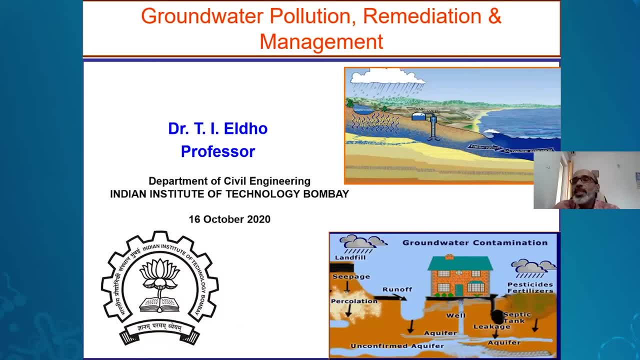 for the entire research community in the country. And now, though, I am not a chemical engineer, but I work in the area of environmental engineering, and, of course, pollution is one area in which I work. And then, today, we are going to discuss. 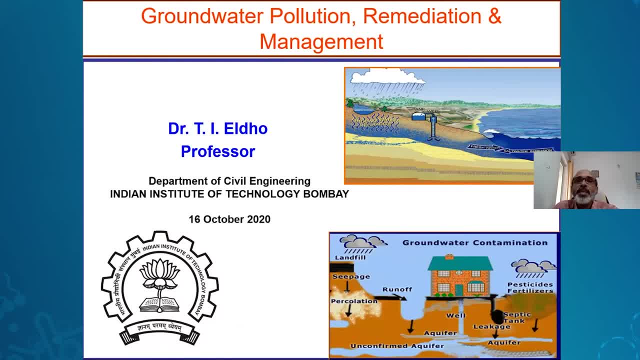 how our water resources can be polluted. So I understand many of you may be chemical engineers or chemists. So, with respect to this, some interesting aspect is that, since everybody- the main connection is that everybody uses water, so I would say how our water resources, or the water we drink, can be polluted. 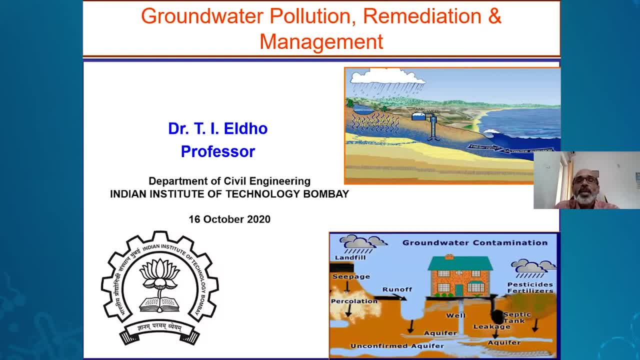 And then as engineers- as chemical engineers or chemistry or bio engineers- what we can do to develop innovative techniques to address the remediation, groundwater pollution issues: remediation and management. So this is what we are going to discuss in today's lecture. 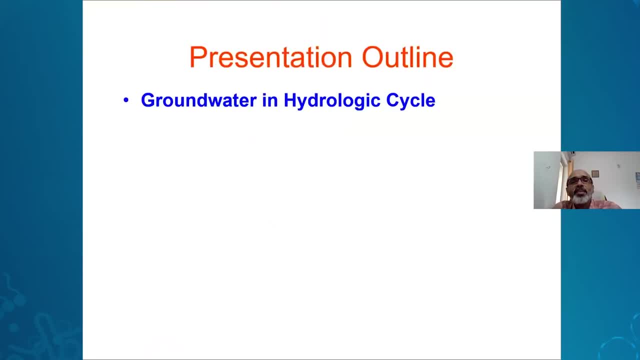 So I will be having around 40 minutes lecture And then around 20 minutes we can have a discussion. So my presentation outline includes So. many of you may not be from the groundwater area, So I will have a brief introduction about groundwater. 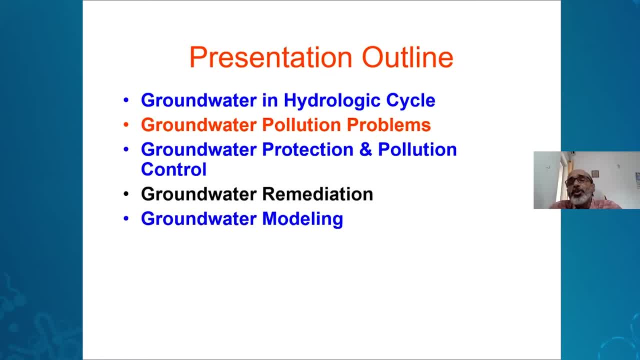 And then we will discuss about groundwater. We will discuss about groundwater pollution problems, Why groundwater is so important, And then what are the sources of pollution, How it is polluted, And then as a common man or common, say, person, 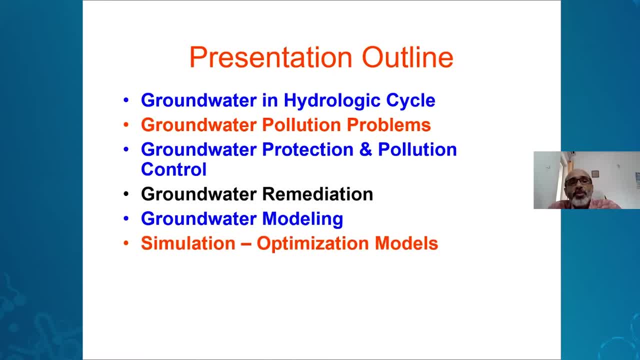 how you can protect your groundwater. So, since most of you, I am sure that, other than cities throughout the country, everybody will be having their own wells and then they will be using directly the groundwater. So how we can protect the groundwater and control the pollution. 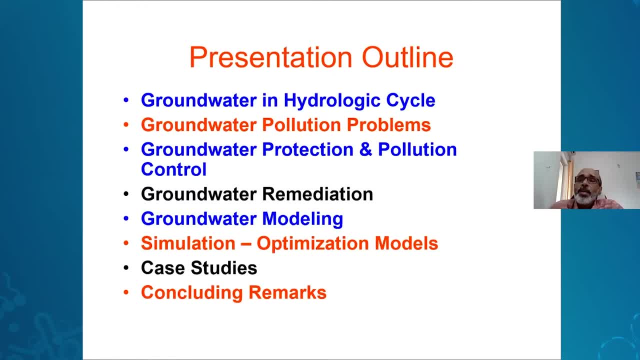 And then say, of course you see that many parts of the country and then many countries say like, especially Europe, Germany, Germany or America or other countries, groundwater pollution is a major issue, since so much of industrialization took place in, say, after 1950s. 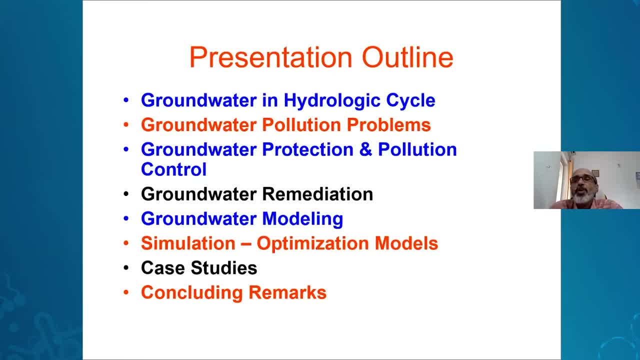 And then this has led to a lot of pollution problems, especially water pollution, And that is especially groundwater pollution. So we will be discussing how to, What are the remediation techniques available And, as scientists and engineers, what kind of technologies we can look into. 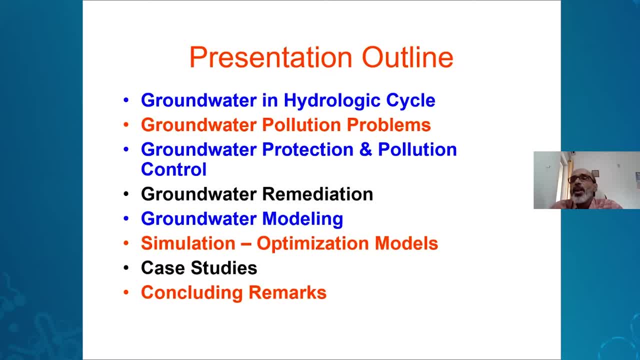 And then, of course, since, as a civil engineer, I am a modeler also, So groundwater modeling, how we can do modeling, some mathematics, how it can be done. And then I will be presenting two case studies: How, if an area is polluted, how much money to be spent. 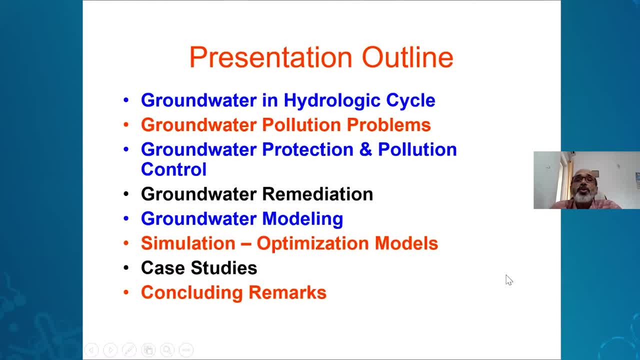 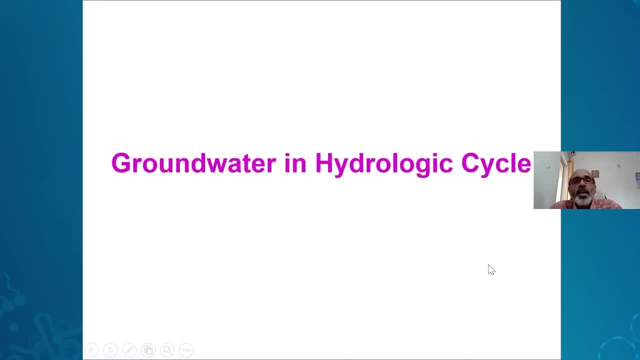 how much time is to be spent. This model, these case studies, will show how the situation and what kind of things we can do. So that is what we are going to discuss today. So I am sure that all of you know what is a hydrology cycle. 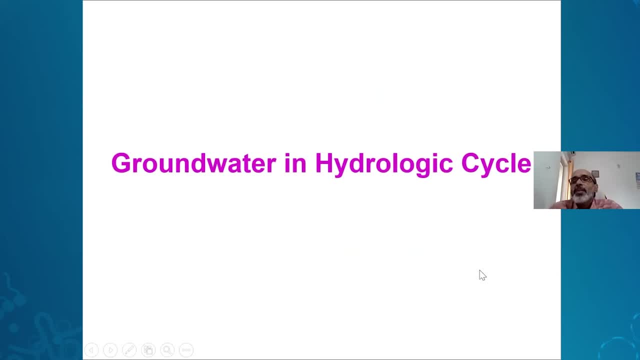 So you see that water is consented. So whatever the water available on the earth it is, will be going, as say, it will evaporate and then it will be coming back as a precipitation, And this is a cycle. So we can see that this groundwater is also part of this hydrology cycle. 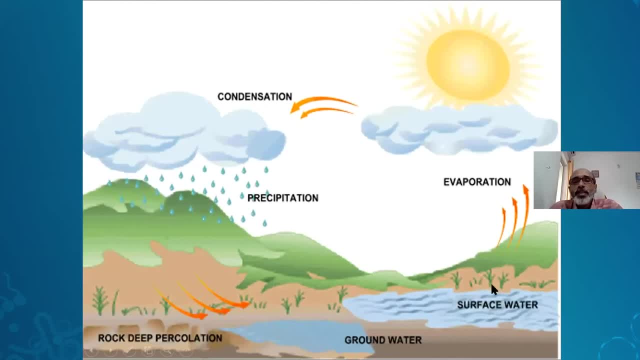 So here you can see in this figure what is happening. So this is a cycle. So here you see that once the water is evaporated, it will be, say, again going further in a cyclic mode, as a condensation, and then it will be coming as precipitation. 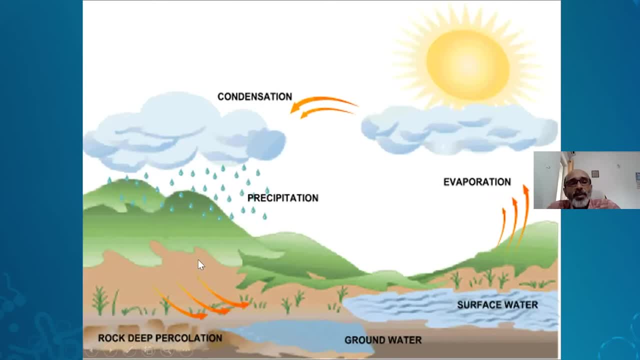 And then it will be some water will be penetrating down, percolating down and then we call this aquifer system. That is what is so-called groundwater And that will be going down and it will be stored. So we say groundwater is a water bank. 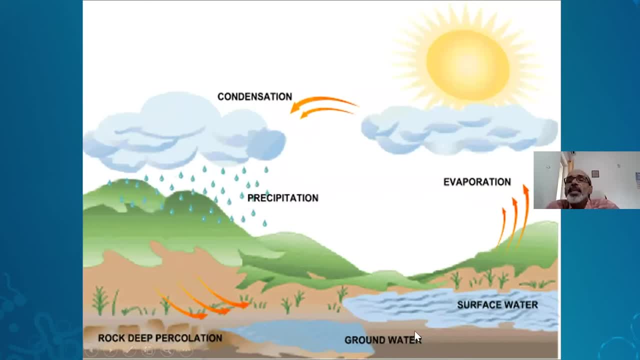 So, like we deposit money in the bank, whenever we need, we can take it. So similarly, we can store a lot of water in the ground and subsurface, So there and then that also, that water is also moving. 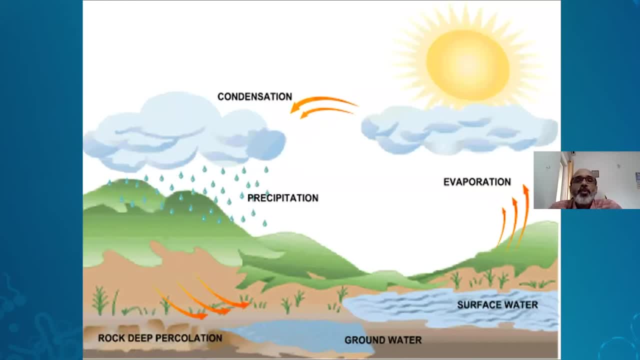 And then we can take it back through wells or borehole, bore wells, all those things, And then some part of the water will be going as runoff and that will be coming as surface water And then this water again joining back to the sea. 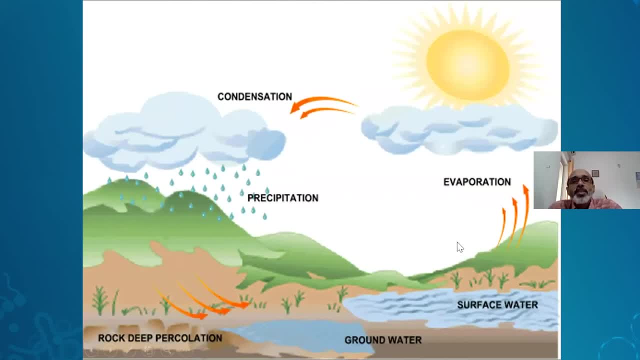 And then that cycle will be repeated. So this is in hydrology, we call it the same Hydrology cycle, And this groundwater is an important component of the hydrologic cycle. So that is what you can see in this slide. 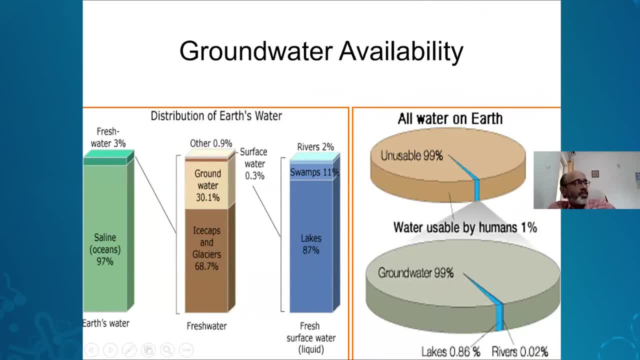 So now why groundwater is so important. So I am sure that many of you are using the groundwater, But you do not know. it is a very important source. So you see that we look at the water availability. So all of you know that fresh water is hardly 3%. 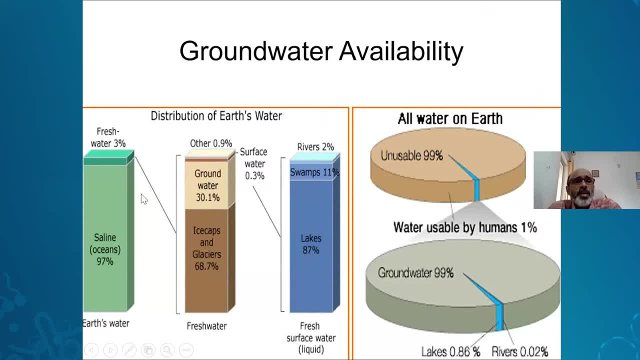 and then remaining 97%, This saline or other kind of waters which we cannot utilize And then out of the fresh water available. So almost 68% is in ice cap and glaciers And then 30% is in the groundwater And then surface water is only hardly 0.9 water. 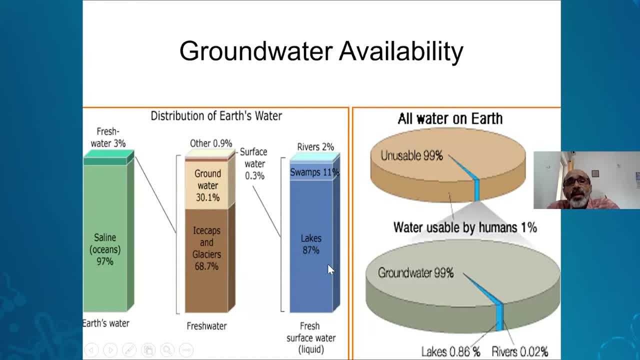 And then available water. out of that again, if you come into this thing, So here. so that way, if you put into, almost 99% of the water is unusable And only 1% is available, And out of that that is the importance of groundwater. 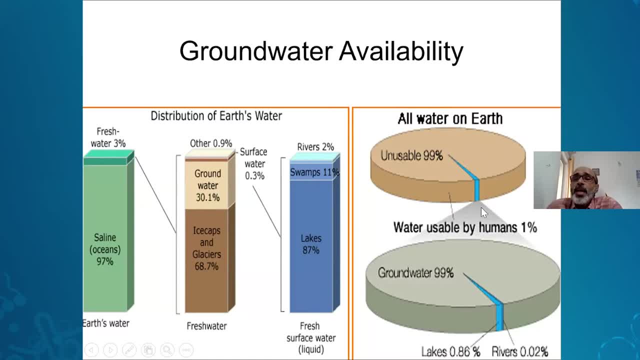 Out of that, 1%, even 99% of the water is groundwater And only hardly 1% is there what we can observe really in the lakes, rivers, like that, surface water bodies. So that is the importance of groundwater. So groundwater is a very important water source. 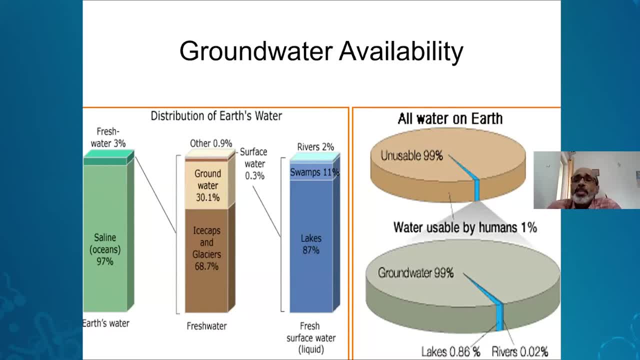 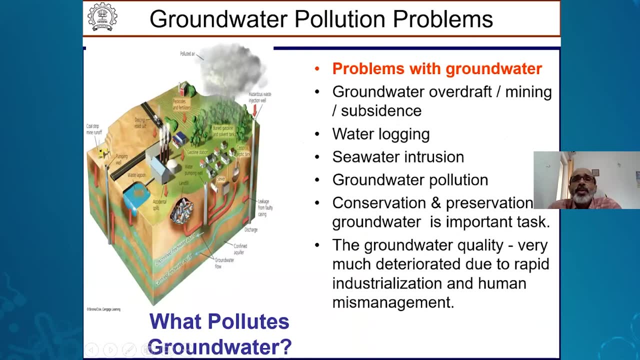 And then many of the plants also get water. Most of the plants get water through groundwater source only, So that way we can see that this groundwater is so important. So now, as I mentioned in, till 1970s and 1980s everybody thought that groundwater is a very pure source of water. 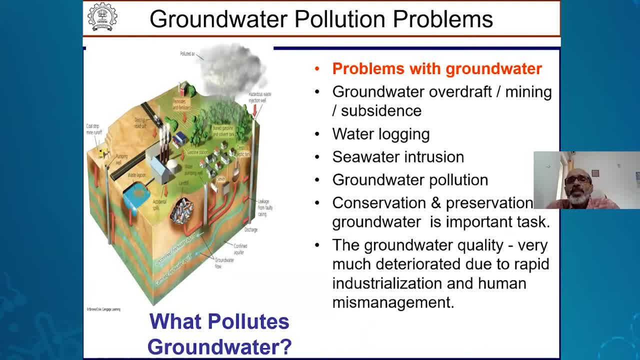 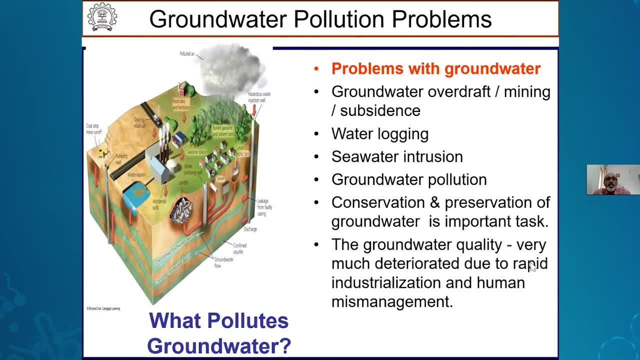 And then. so nobody bothered much about groundwater. So that way, now if you look into this, what are the problems as far as groundwater is concerned and groundwater pollution? So now, if you could look into groundwater, what are the important problems? 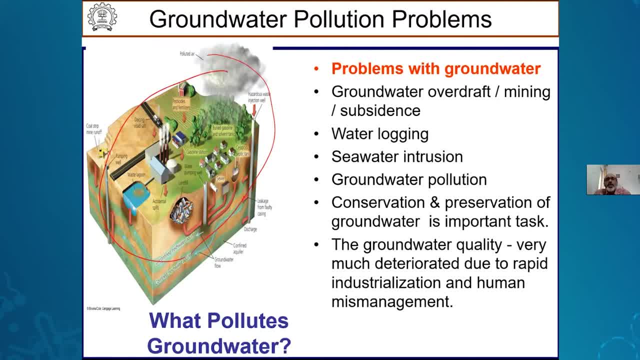 So you can see that there is so much of the problems are there? So one important problem is quantity is concerned, Groundwater overdraft. You see that those are in India. You could see, you would have heard about the so much groundwater is drawn in Punjab, Delhi region. 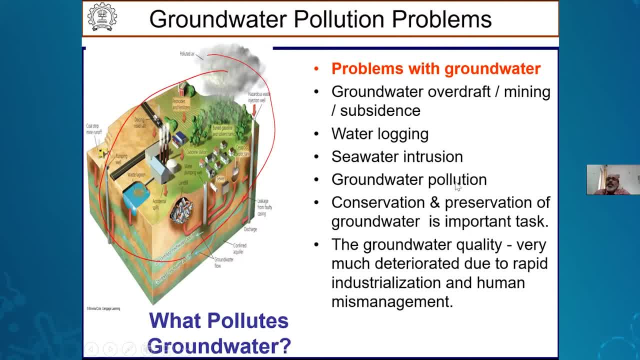 And then it is going drastically down. So farmers are putting their wells with 900 feet or 100 feet down and then trying to extract water. So that is a major issue in many areas. But some area of water logging is a problem. 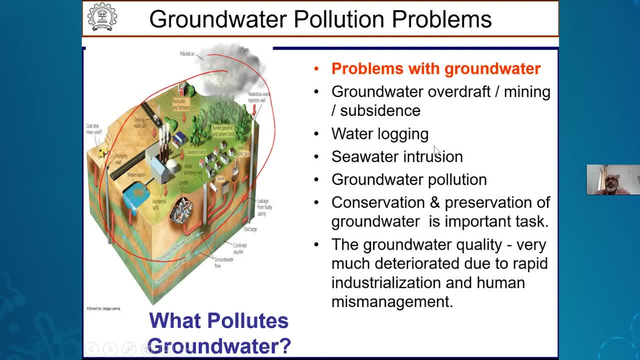 So you see that water logging means already the surface, already too much water is there, And then we cannot use that area for even for farming. And then coastal region: there is a sea water intrusion problem is there. So that is another problem. 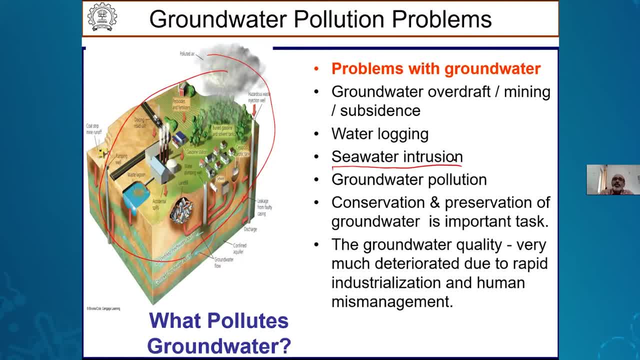 And then. so that is about this, That is about the general issues are concerned. Now, coming back to so much, groundwater is available, but if it is not good quality, then it is useless. So that is: groundwater pollution is a major problem. 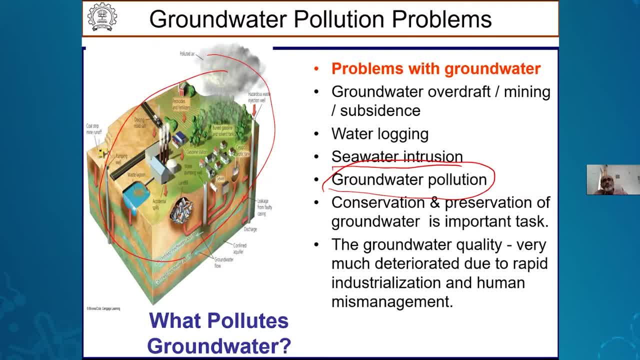 So we need to see within this context we have to conserve, preserve the groundwater, So it is so important. So I hope those who are hearing me, all you understood what is the importance of groundwater, Why we need to protect the groundwater. 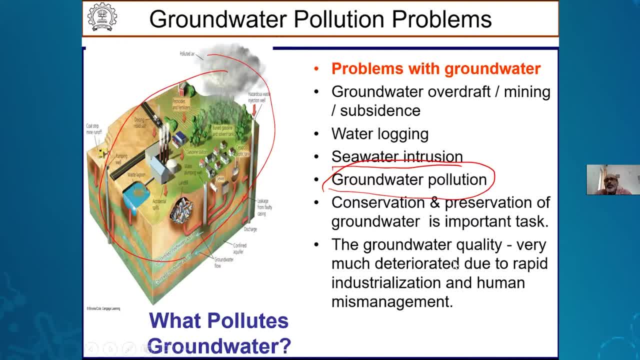 And what are the pollution problems? So groundwater quality is much due to rapid industrialization and human mismanagement. We have to say this mismanagement Since we are controlling the many things and then we are not doing things. many places, Like if you go to Patanjali near Hyderabad, or if you go to Palar in Tamil Nadu. 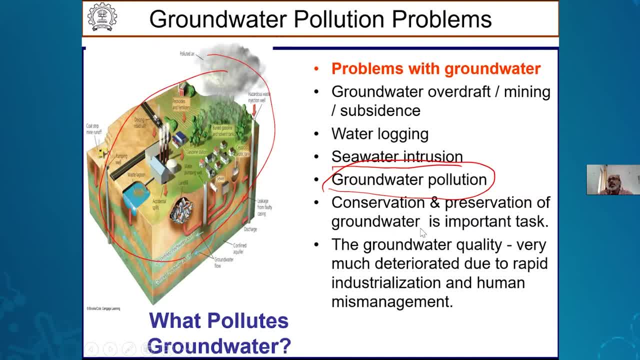 Many locations you can see that so much of the industries. they did not flow properly And then they simply deposited this. They are affluent in the either underground or in the surface water itself And these are all causing the big pollution. So that way, when we look into, let us see what are the contamination sources as far as groundwater is concerned. 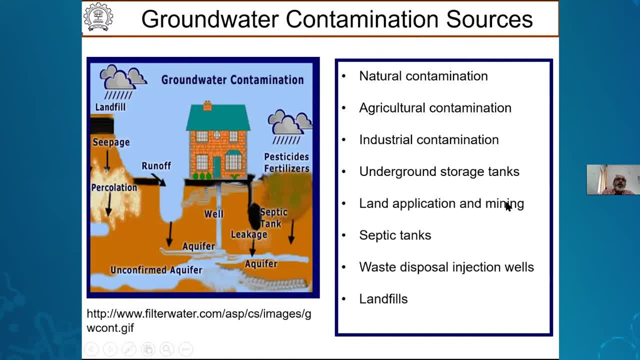 What are the contaminant sources. So here this figure shows what are the important source of contamination. So you can see that it can be We ourselves, like whenever we are putting our human excrete, all those things. If there is a leakage then that can say pollute the groundwater. 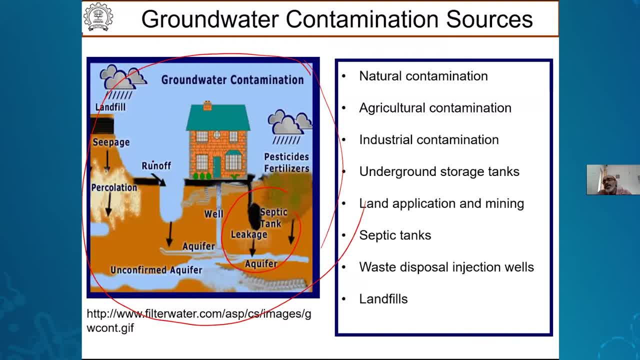 And then also say if you are putting dumping anything on the surface. So nowadays monsoon, Now monsoon is ending, So these water bodies we are putting that will be coming going to the surface water and then groundwater. And then farmers are concerned. they use lot of pesticides and fertilizers. 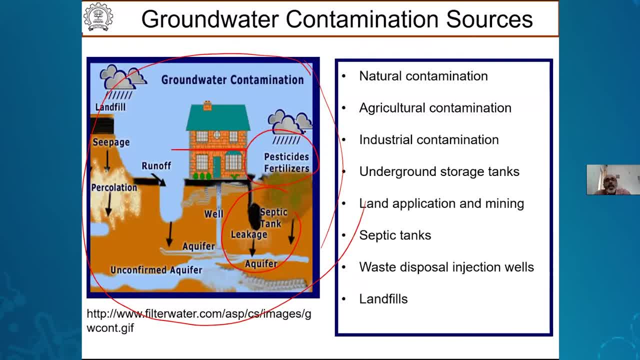 So this: you can see that slowly penetrating down through the soil And that will be that is also called a distributed or non buoyant source of pollution. And then, if many industries use their underground tanks, like especially in petroleum products in India, still we are using underground tanks. 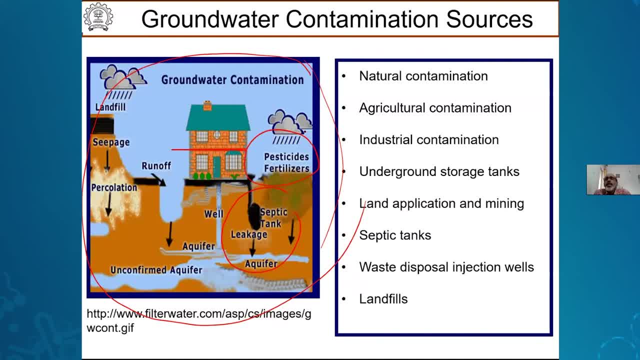 So these tanks may be having lot of many places, lot of leakage And that can pollute the groundwater system. And then you see that in many locations landfills are there. We use it as a. If you ask an environmental engineer, then the landfill is a major source of 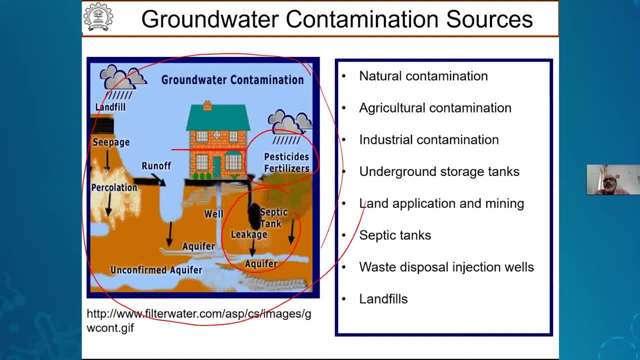 Like we Dispose the waste through landfill, So that you can see that leachate will be produced And that will be slowly penetrating down to the aquifer system or the groundwater system. So that way we can have, And natural contamination means you see that arsenic. 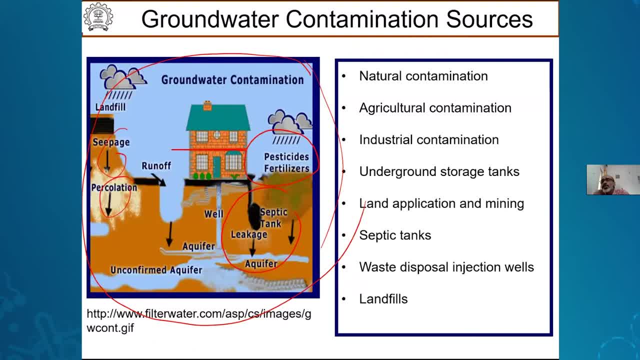 You can see in Bengal belt there is an arsenic problem. So much groundwater is extracted That region. it is naturally happening, And then also sea water integration. So that is natural way of contamination. So important contamination source are natural contamination, agricultural contamination, industrial contamination, underground storage tanks, land application and mining, septic tanks, waste disposal, injection mills, landfills, etc. 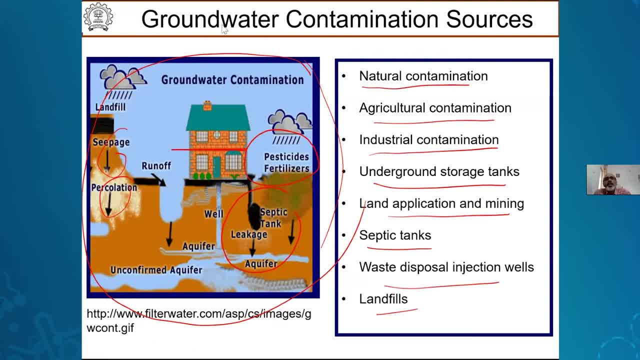 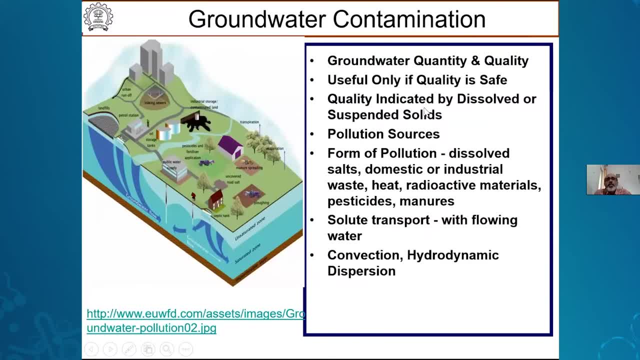 So these are some of the important sources of contamination, as you can see here. So now, if you look into, So, as I mentioned, when groundwater is concerned, We need to see that not only quantity. If too much quantity, then quality is not good. 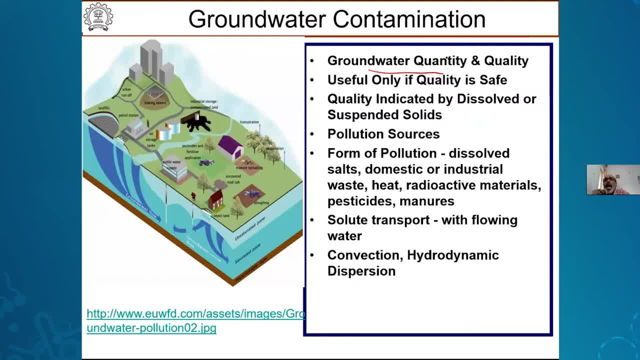 It is not at all usable. So quantity and quality are so important. So it is useful only if quality is safe. So that is very important And quality indicator generally. As in the, many of you are chemical engineers or chemists. 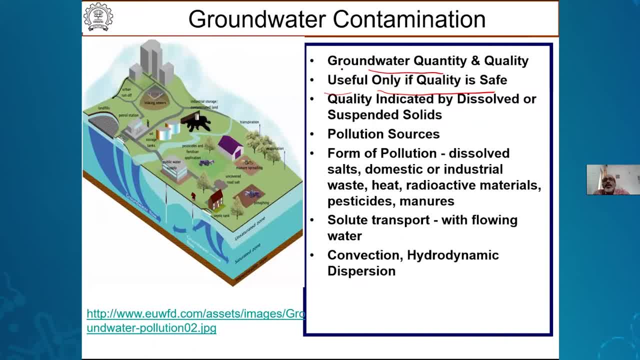 So you can see that quality indicator generally by dissolved suspended solids. So that way and depending upon the pollution sources. So here again I have a number of pollution sources. So it can be this pollution can be in the form of dissolved salt. 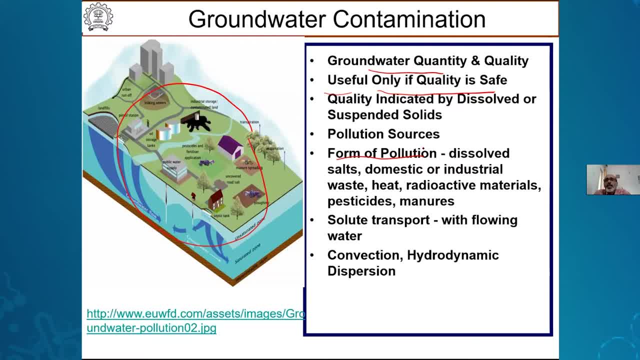 domestic or industrial waste, heat, radioactive material, pesticides, manures, etc. So these are the way the pollution takes place, And then we look into this pollution, how it is going through the water. There are different ways the processes are there. 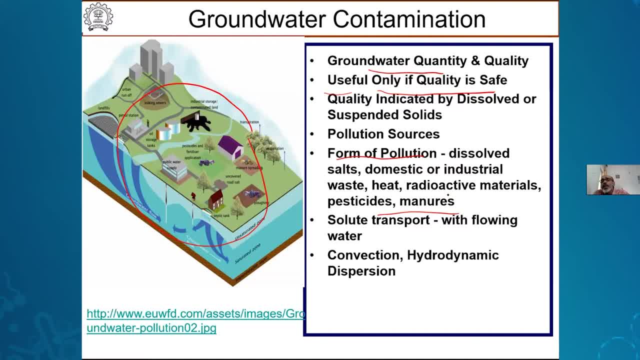 One is diffusion, of course. diffusion, Then advection or convection, and then hydrodynamic dispersion. So this is what processes that will be taking place once this contamination goes to the groundwater. Then it will be slowly spreading, like this. So that is what you can see. 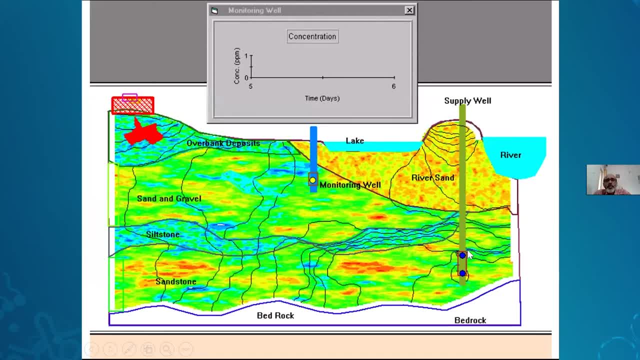 So this animation shows what is happening. So here you can see now this is a landfill And from that the leachate is produced, And then it is slowly coming, And then you can see This is the aquifer system, or this soil system. 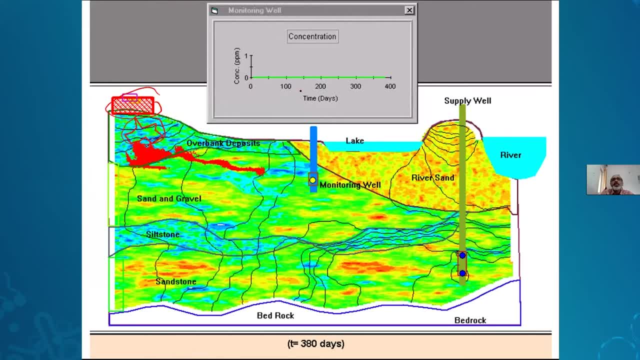 So through that, how it is spreading. So here you can see time versus concentration is important in this graph here. So now let us assume that here there is a municipal supply there, say, for example. So how it is reaching, So you can see that it is now after 600 days of this. 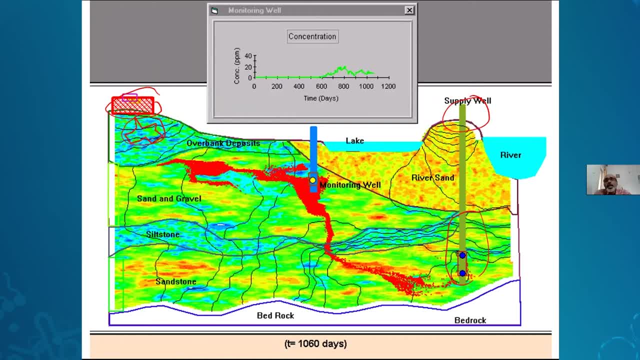 So here the supply well is getting the contamination. So that is the way this movement takes place. So that is a very, very, very complicated process, So it is not a one-in-one. One important thing is that nothing is visible. So that is our major question. 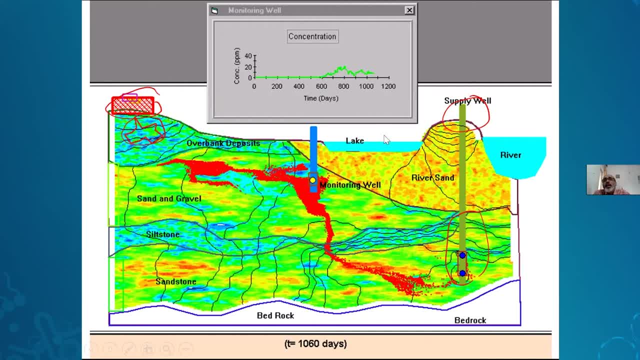 So we need to put in so much of assumptions and then see what is happening. So that is why we have to be very, very careful. Especially the engineers have to take leach, See that we shall not pollute even the soil, or we should not dump the waste like that without scientific landfilling. 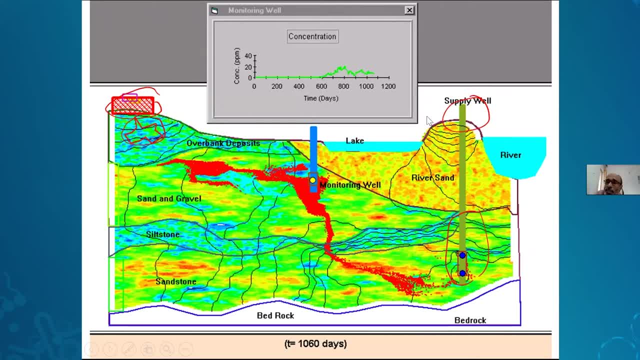 Or we shall not put the any kind of solvents like petroleum in tanks which there is a possibility of leak. So that is what you can see, that now, finally, contamination is reaching to the well, And that will create a lot of problems. 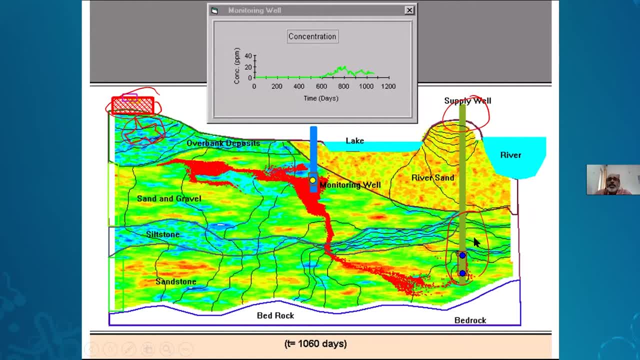 And this is really realistically observed in many parts of the country and many parts of the world also, So that you can see: So that is what is happening, And now you see that the system is so complicated. So, as I mentioned, the soil is concerned. 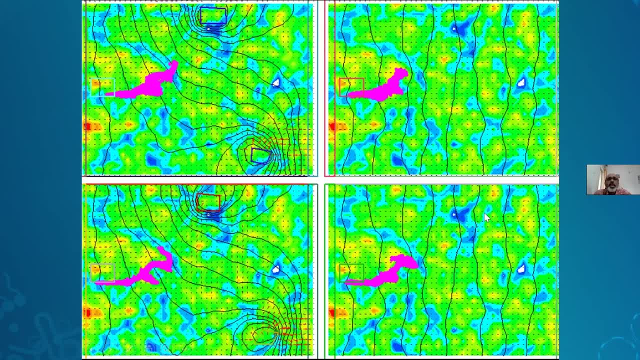 All of you know that aquifer system, Soil for the porous media is concerned, It is so complicated system So it depends upon things We do not know. So one feet and the feet Say one foot and the foot, or the one centimeter, tiny centimeter soil is so heterogeneous. 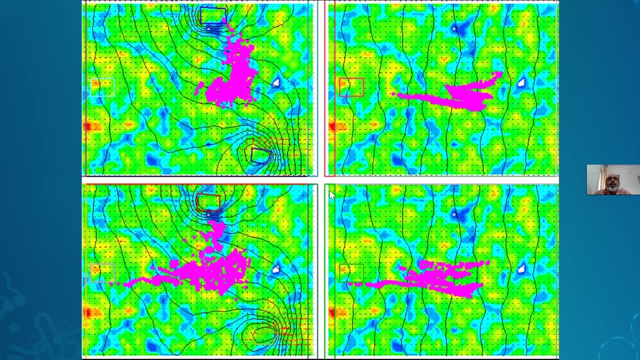 So that we do not know what is realistically happening. So for modeling sake, we put a number of assumptions, number of simplifications, But you can see that what is happening here, Say, if a contamination from this, how it is moving Some places, it will be fast moving. 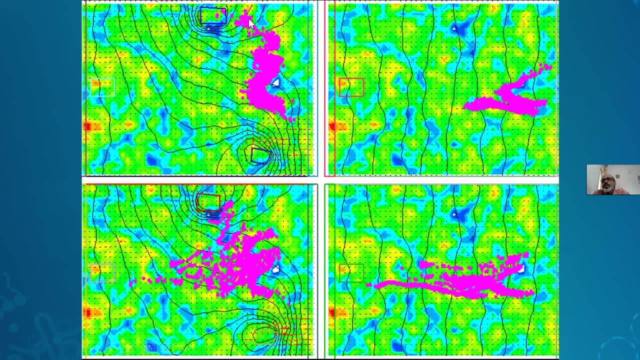 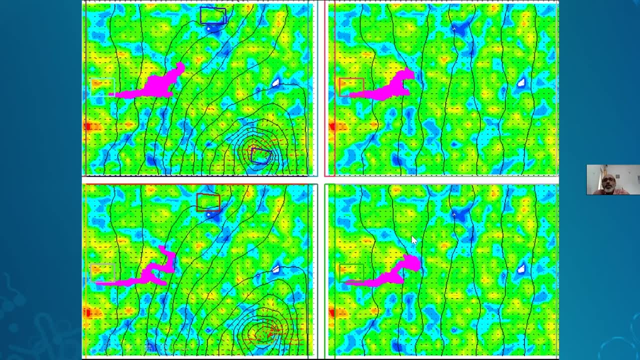 Some places very slowly moving. So, depending upon the soil, heterogeneity, Then anisotropy, So the system, variations can take place, as shown in this animation. So these are all the major kinds of issues. So here you can see, for example, this animation from one produced in US. 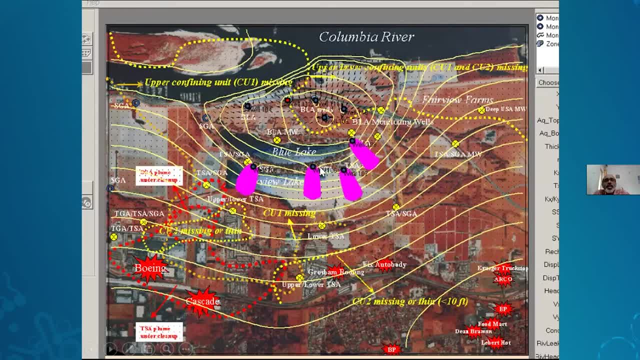 So Columbia River is going. Now you see that these are pumping well, And then how much area it can affect when you are pumping water from a particular area. So you can see that these are the influence zone. It can be hundreds of meters influence zone is possible. 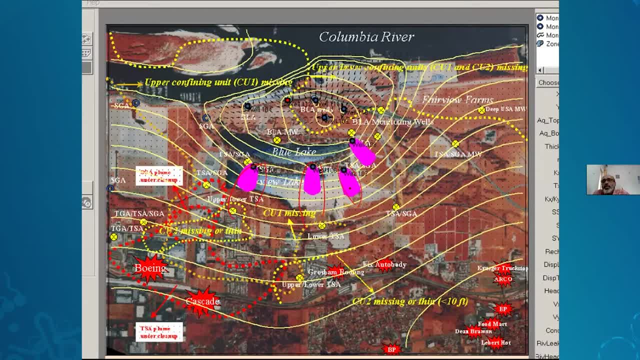 So that way, if nearby areas are there, Then it can also have this contamination that can take place. So that is what we can observe in all these problems. So this 2-3 animation shows what are the major problems And how so complicated or how complex is the problem. 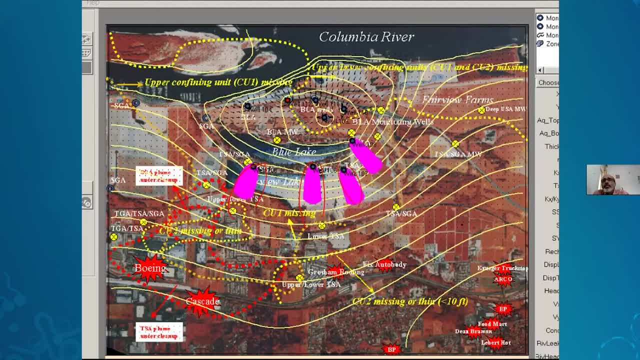 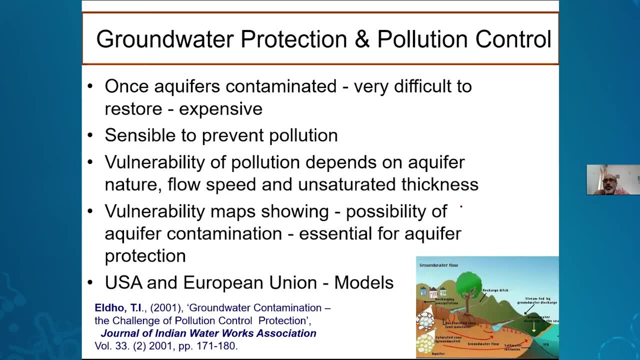 And that I hope all of you understood. Now, coming to Now, let us see how we can protect and how we can control the pollution. So, being engineers, we need to see that It is how we can do even your own well. So if you have a well in your land, 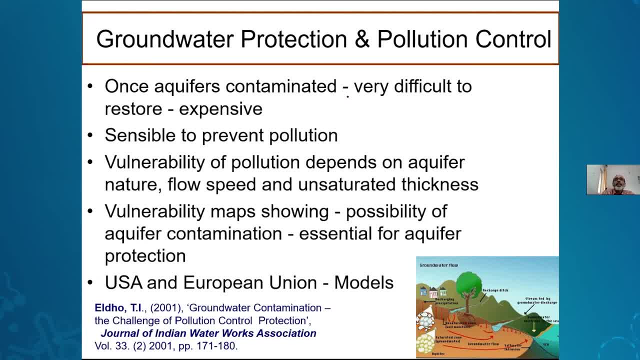 Then how we can protect it. So once aquifer is contaminated it is very difficult to restore. It is highly expensive. The last case studies which I will be presenting You can see that how much expense and how many years we need to do the treatment. 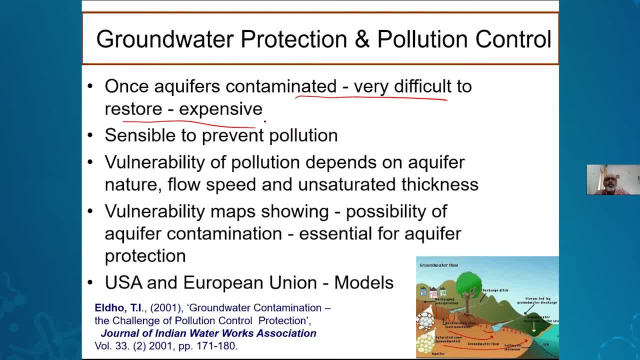 So you can see that. So it is always sensible to prevent pollution. So that is groundwater protection. We always propagate, And vulnerability of pollution depends on the aquifer nature, Floss field and the unsaturated thickness. How much is unsaturated thickness? 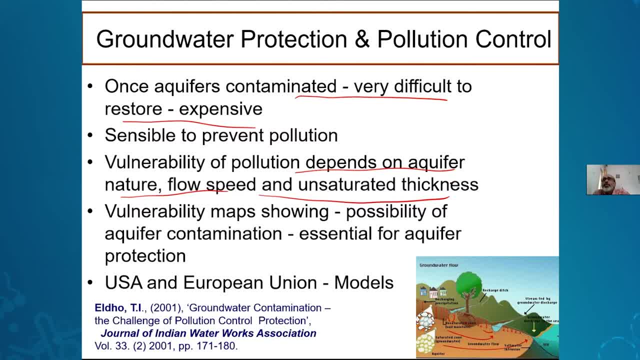 All this depends upon that And we can. So if you are municipality or if your area, lot of water is there, Especially for municipal supply, If you are pumping groundwater, So then we need to see that We can prepare vulnerability map. We can see the possibility of aquifer contamination. 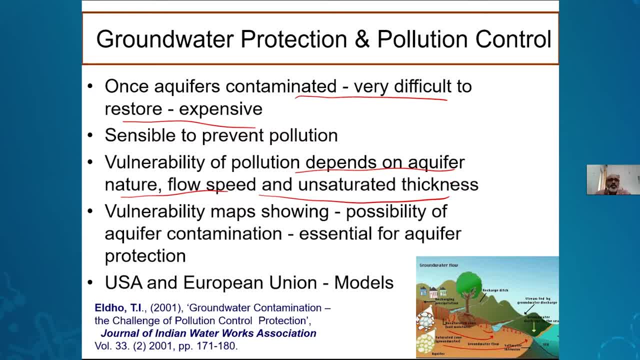 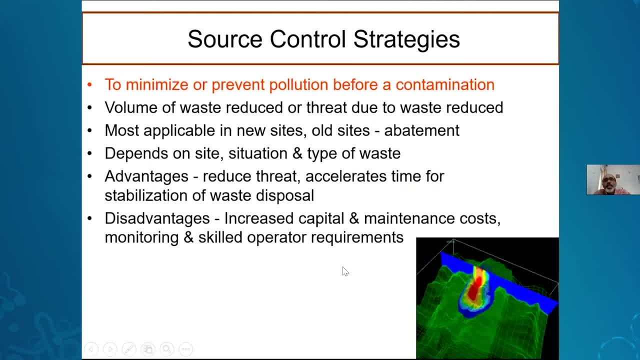 And then we can say that the areas we can protect. So there is a variety of models Like American and European Union models are available. So generally many places like Germany, They use so much groundwater, So there they protect the system with various sonation practices. 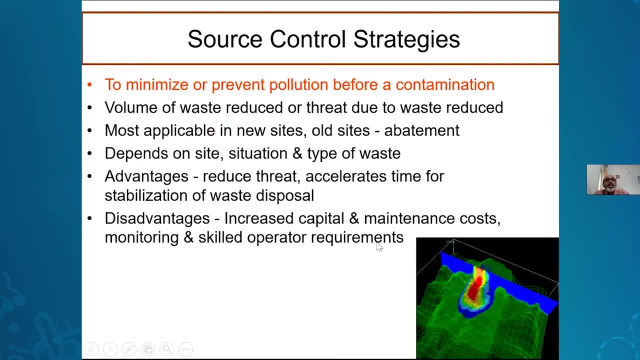 So that I will show you. It is coming in the next slide. So now, if you have got a landfill, Or if you have got some, Now the pollutant is there. So then, how? What are the source control strategies? So that is very important. 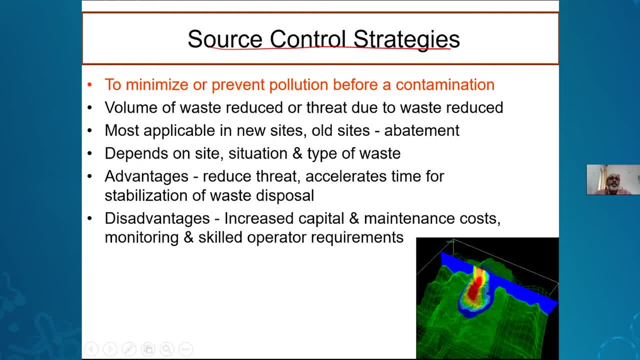 So to minimize or prevent pollution before contamination. So we can see that various techniques are there, Like volume, waste we can reduce, And then, most applicable in new sites, Like all the sites, abatement only we can look into. So this depends upon how much the volume can reduce. 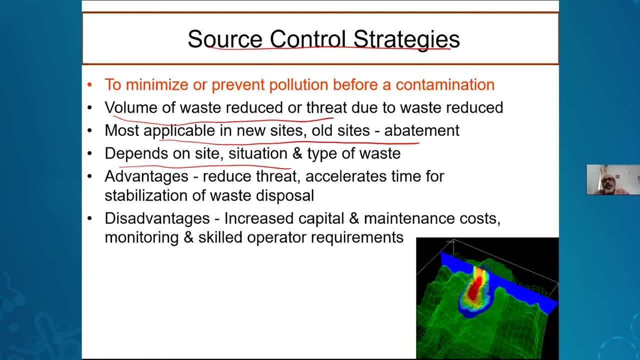 So depends upon site situation, type of waste, etc. The advantage is that this reduce the threat, Accelerate time for stabilization Of waste disposal. So that is what we can see, But many times it is difficult to increase the capital. A lot of money to be spent. 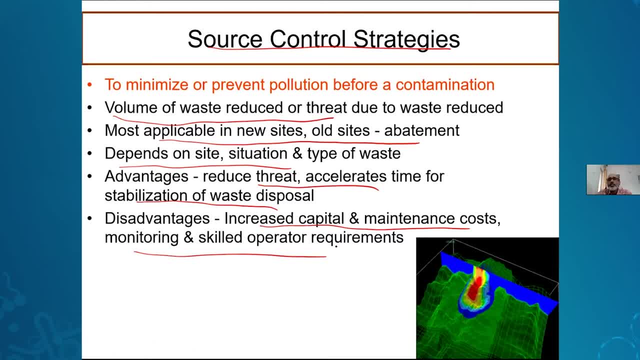 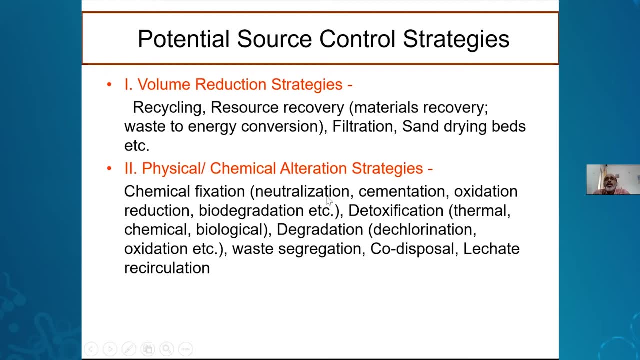 And then we need to monitor, And so here, if it is there, How much it is spreading, We need to see the soil And then how the spreading takes place. So that is also very important. So that way some of the potential source control strategies. 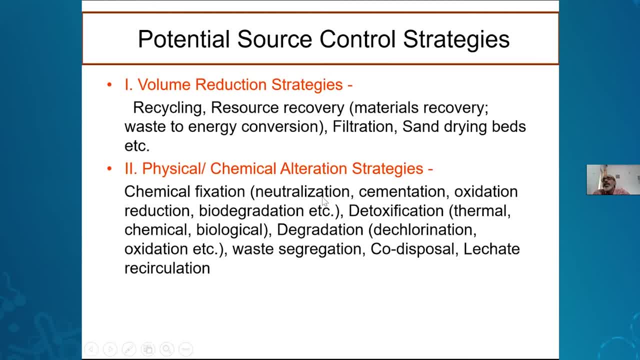 So in India that much research is not taking place in the area, So there is a lot of scope for research. So one technique is like, as I mentioned, Volume reduction strategies, So we can reduce how much is the pollution Or how much is the waste. 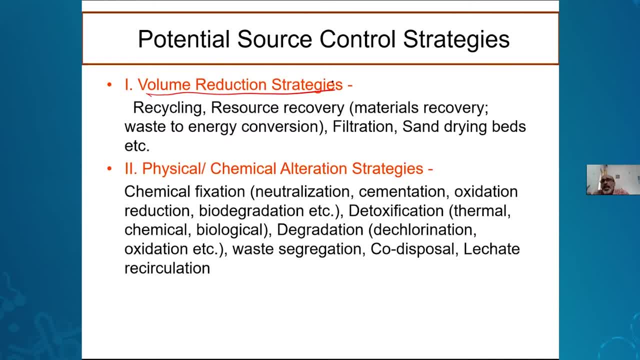 So there is all of you know. We can do recycling, Like plastic recycling Or any kind of recycling is possible. Then we can go for resource recovery, Like material recovery, Waste to energy conversion, Filtration, Sand drying, etc. So there is a variety of methods. 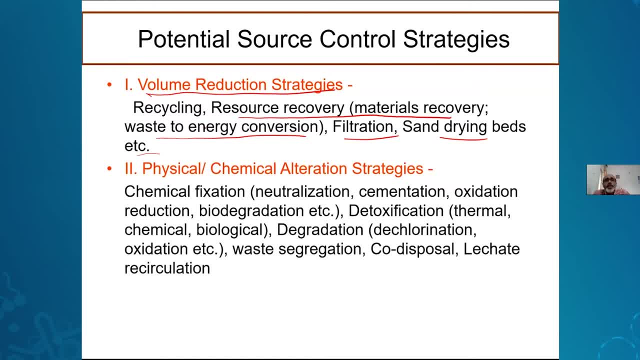 For volume reduction strategies are there, And then comes physical or chemical alteration strategies. So this is especially being Since I am talking to mainly chemical engineers, So their chemical alteration strategy is very important, So we can chemically fix the contamination, So like neutralize. 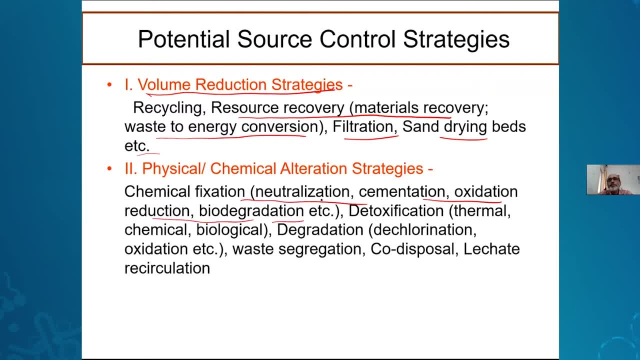 Cementation, Oxidation, Reduction, Biodegradation, etc. Then we can go for detoxification Using thermal technologies, Chemical, Electrical technologies, etc. And then degradation, So we can degrade the waste Through various means, Like by using chlorination. 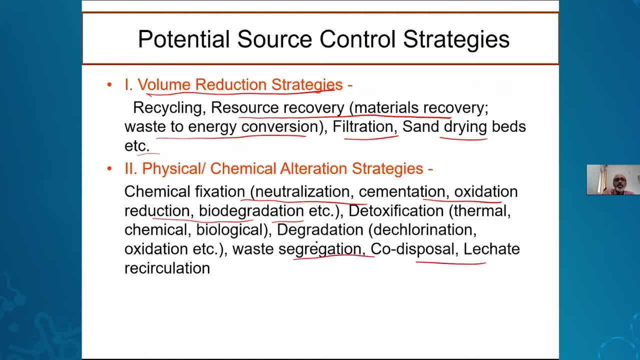 Dechlorination, Oxidation, etc. Then waste segregation, Co-disposal, Re-circulation, So there is a variety of methods As far as physical and chemical alteration strategies are concerned. So, as I mentioned earlier, So there are European Union and American models are there. 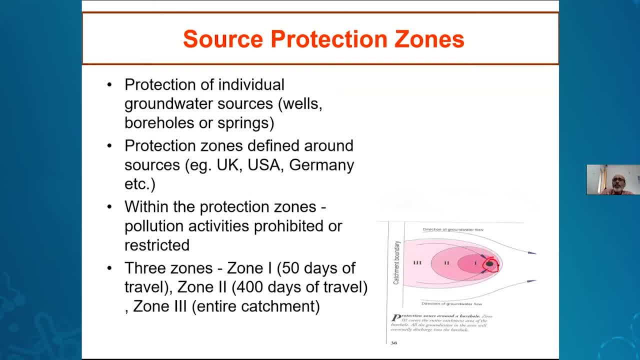 So, for example, What do these models say? So here we have got a pumping well, So that is, a large quantity of water is pumping. So, generally, what do they In their system? What do they do? There will be three types of swarms. they will be defining. 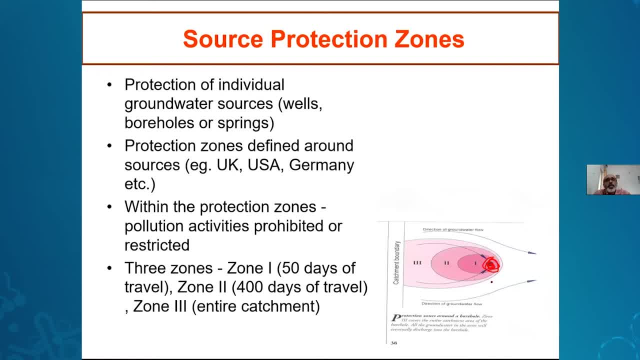 So we have to protect the individual groundwater source like wells, boreholes or springs. So here through numerical simulation we can identify which is a critical swarm. Like three swarms, One means 50 days of travel of water, So that is, This is so called a swarm 1.. 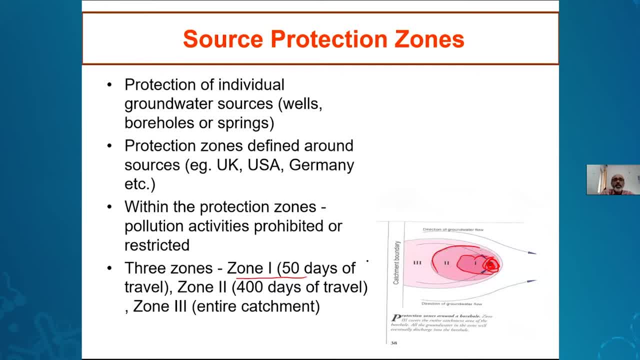 And then 400 days means swarm, 2. And then swarm 3. The entire catchment. So, for example, if a well is there, That aquifer system, The entire catchment. So there A variety of source protections, Say, for example, if a particular groundwater well is there, especially for municipal supply. 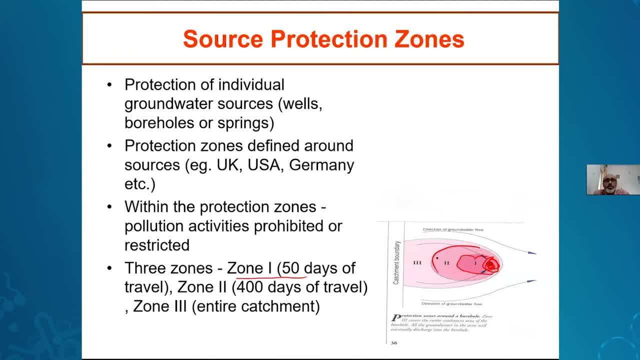 So they restrict all kinds of development in swarm 1. So that is where 50 days of travel is there And swarm. 2. Restricted development only allowed And swarm. 3. Of course some control, like chemical industries or all those things are controlled. 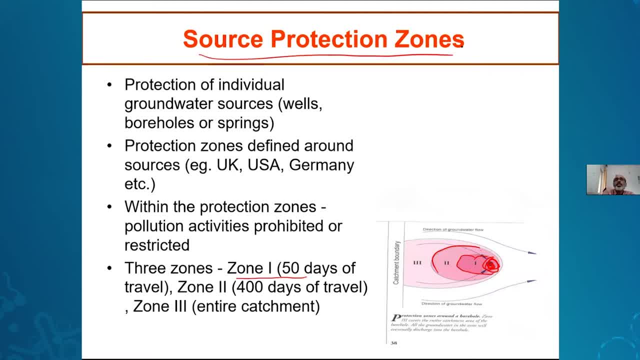 So that is the way We do the source protection, Source As far as the groundwater protection is concerned. So now, Like, since I am talking to chemical engineers, So there is other kinds of technology, Once the Like in a landfill or other areas. 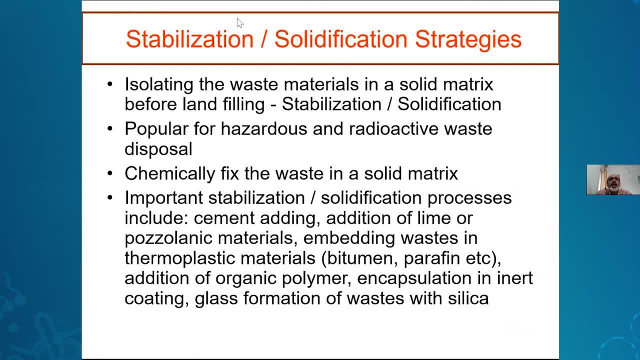 So we can. This waste is contained. We can isolate the waste material in a solid matrix Before landfilling or stabilization or solidification. Then popular, hazardous and the radioactive waste disposal are there. So then we can carry on. We can, We can. 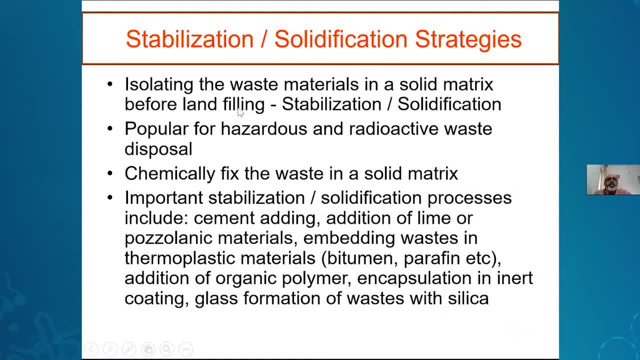 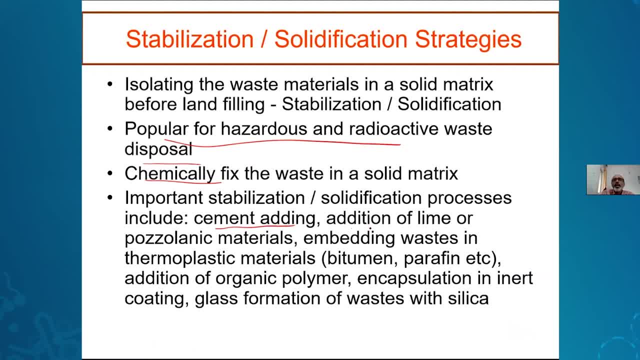 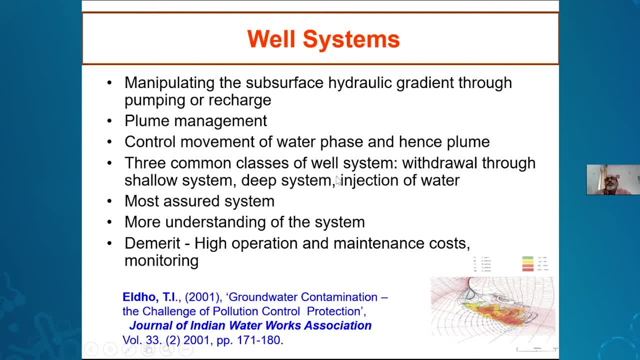 As far …. Algasadation, Since I am a civil engineer, So you can also use Well systems to protect Especially. They pump water well from where we are pumping, so you see that this is a contaminant room. is adding the. 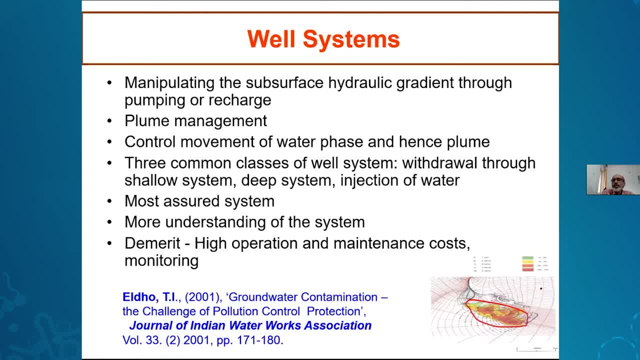 fire. you can see here and now. let us assume that we have got a pumping well here, so then we can use, say, either an annual infiltration well or another kind of the way we are pumping, so that that all those things can be controlled by variety of ways. so that is. we call it this. 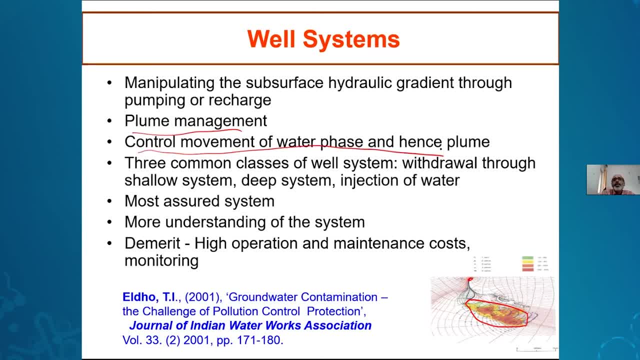 room management. so control moment of water phase and hence broom. so that is, i mean, the movement. so if we are pumping well here, so instead of going to this we can make such that it is slowly moving in other direction. and three common class of well system: like we travel through shallow. 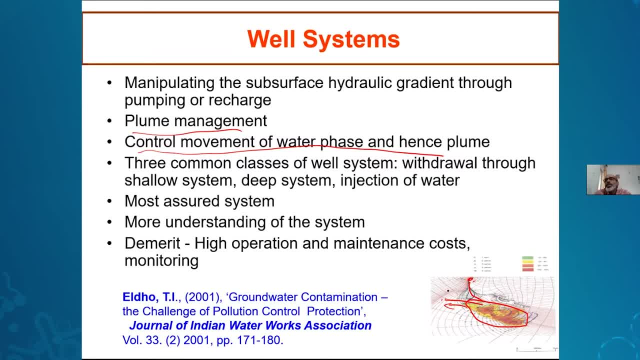 system, deep system, injection of water, so like that. so this is a, but we need to have a number of observation wells for these kinds of problem, so this is the most assured system. more understanding of the system is required. so, as i mentioned, our challenge is that we cannot see what is happening. 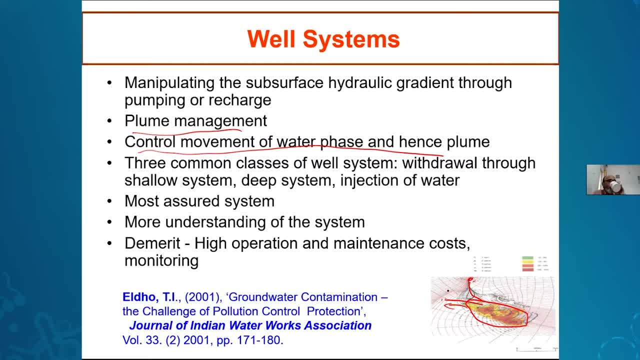 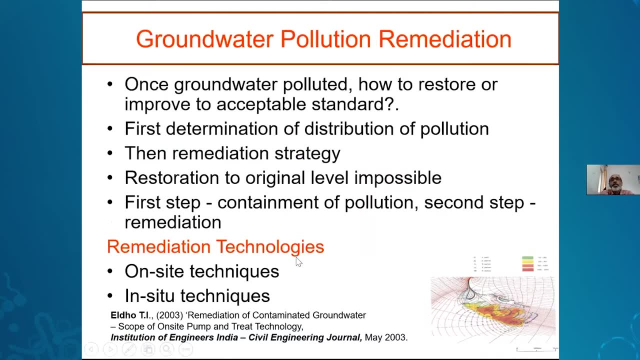 and that is why it is so difficult. so here it is a moreover. but it is expensive also, since the continuously pumping or recharging, all those things are required. so this is so called we can do the well system. so now let us assume that some area is already contaminated. so now, first thing is that. first thing is that we have to stop. 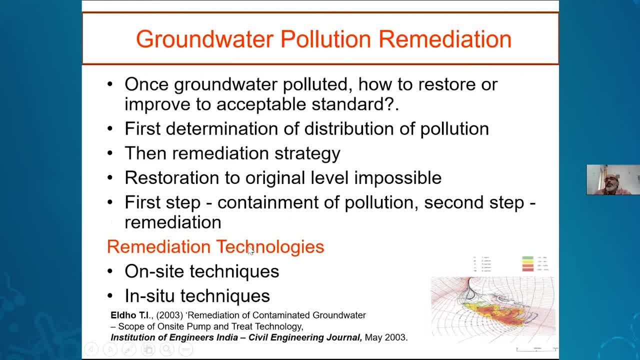 um contamination. so if say, for example, in your region and say a petrol, petroleum, petrol tank which is put in underground, that is, let us assume that that is polluting the, the aquifer system, then first thing is to be done is that we can identify that source and then stop that. so once you don't want to pull it out to restore. so 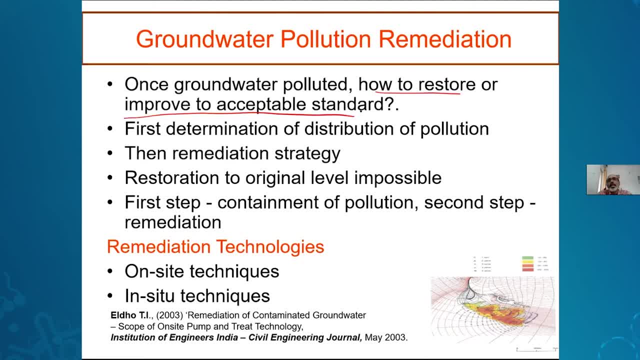 that is what we are mainly discussing: to improve the acceptable standard. so that is the question we need to ask. so a few important steps are there. so first thing is that if you can identify the source- so that is one of the most important step- and then determine the distribution. 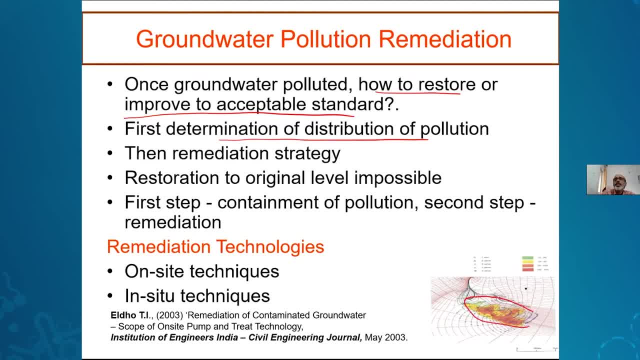 of pollution. so you see that how much area is polluted, where is the plume location, how the width and length of the plume? so all those things we need to look into. so then, once the plume location is identified and its extent is identified, then we can go for remediation. so different kinds of 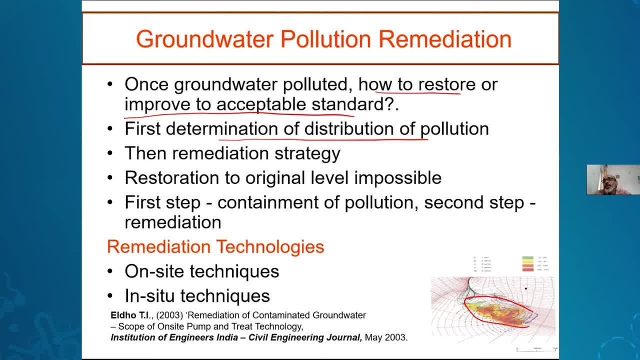 remediation is possible. so here i would like to say that, for example, if the tds is concerned, if 3000 ppm is there, then if we can reduce at least 500 or 750 ppm, that is what we look into. so restoration to original level is impossible. task and first: 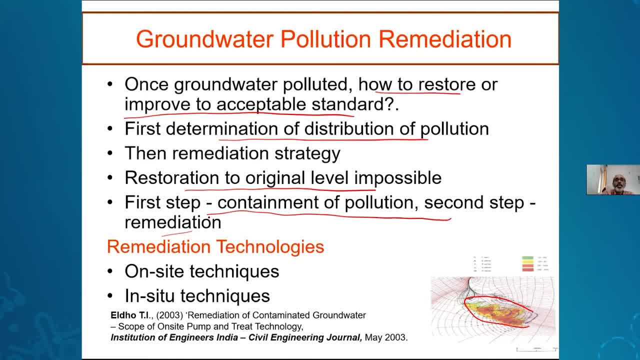 step is to containment of pollution and second step is remediation. so these remediations are concerned on-site techniques are the in-situ techniques are. there is two kinds of remediation technique. one is on-site techniques, in-situ techniques. so on-site means generally we will be pumping out polluted water and then treat it and then we can infiltrate down. 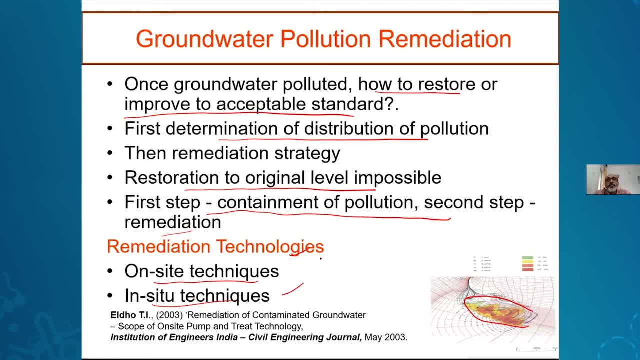 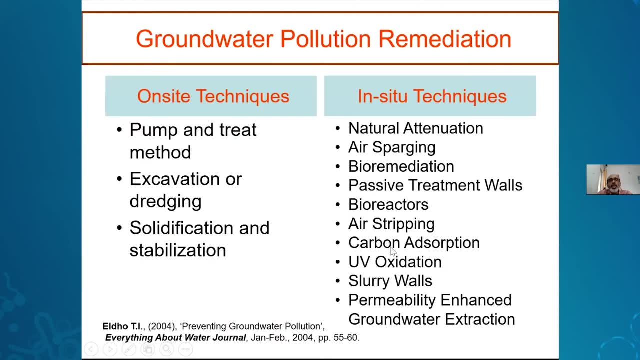 or we can reuse it. that is so called on-site technique. in-situ technique means we are not pumping out the water but through bioremediation or like various kinds of techniques, we will be at the location itself. we will be remediating the polluted water. so that is in-situ technique. so this: 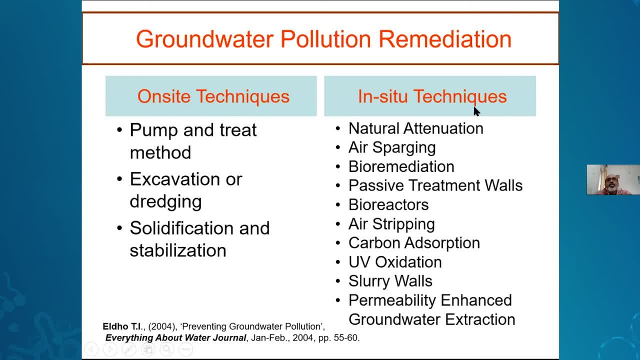 is the. a table shows the difference between on-site technique and in-situ technique. so here you can see generally used on-site technique is pump and reach, so you are pumping the waste water or the polluted water and then treatage, and so then we can use sales. soil is polluted and we can excavate. 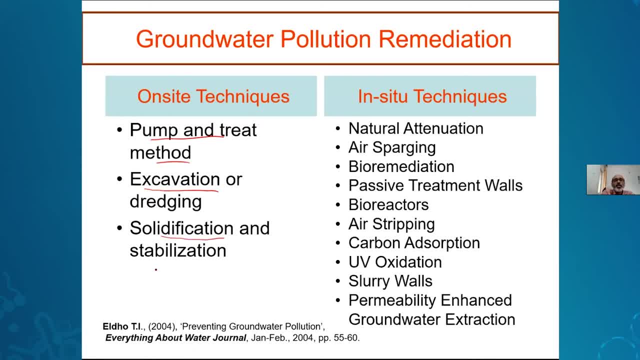 or dredge it, and then we can treat it, and then also we can go for solidification and stabilization etc. so that is on-site technique, institute techniques. so for example, if your land is polluted, so you have got a 10 cents of land, and then if the soil is or aquifer is polluted, then but if you are not using 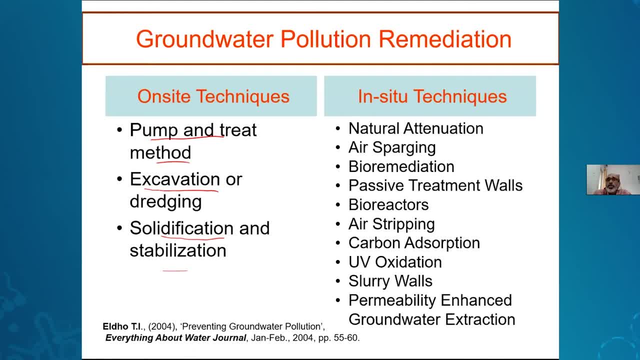 that water. then of course, due to natural means, of course a lot of bacterial activities and other kind of activities, naturally they can get any attenuant, but it will take so many years, maybe say tens of years, or 20, 30, 50, 100 or so years can take place. so let me say, for example, now you all 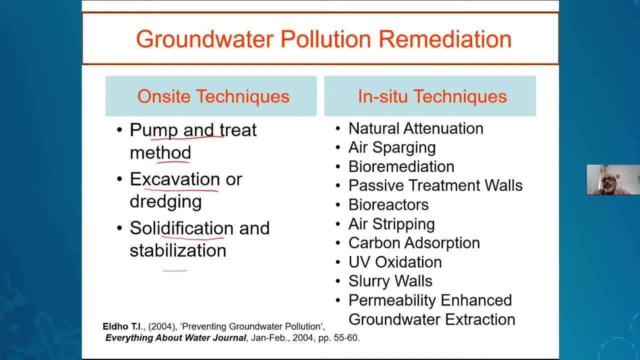 of you know that bhopal tragedy. so that they are uh the, uh medial isocynate or some contamination is identified in that location in the ground water. so still, uh, that water is not using. but now, even after um september, 20, 25 years, you can see that still, uh the the contamination is there. so that is what is. 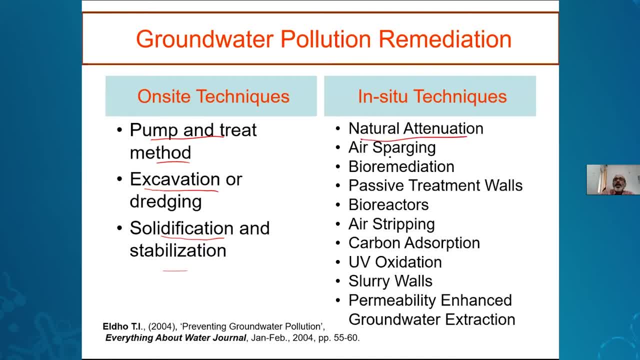 identified. so natural attenuation is a very slow process. then some of the other techniques, like air sparging. so, for example, if it is the your contaminants, organic and dams like petroleum products, so we can go for air sparging, we can introduce air into the system and then, uh one. 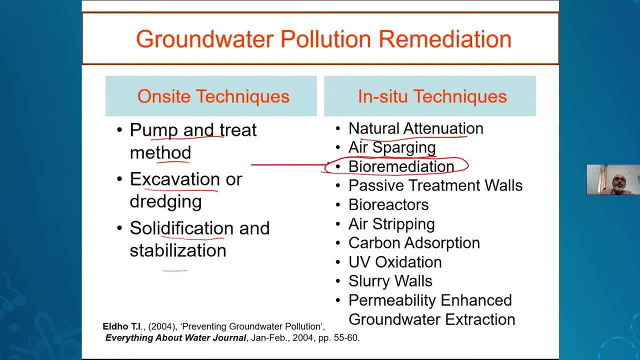 most promising technique where all of us has to look is so called bioremediation. bioremediation means we are identifying the contamination and then we identify certain bacteria and then we allow that bacteria to grow in that area and then that will be eating down. 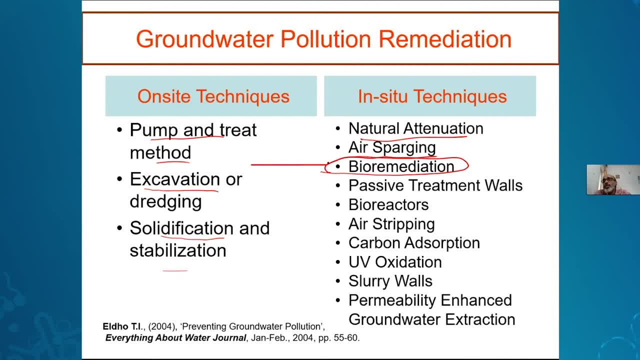 this contamination and then it mainly what is coming out to the carbon dioxide, or just plus water like that. so that is what is the most promising technique in a country like india. so then we can go for other kinds of treatment: technically passive treatment, while bioreactors 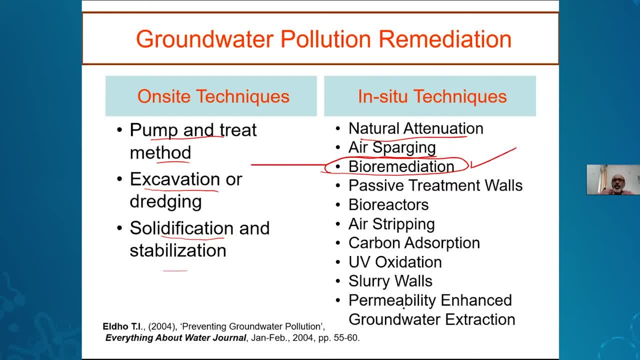 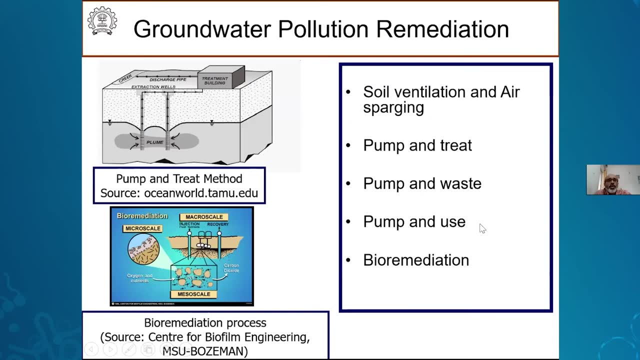 then carbon absorption, uv oxidations are rewards. a variety of techniques are available and many of these techniques are used in developed countries like america, canada or uk or germany like countries. these are all very much used. so some of these important techniques will have a brief overview. so pump and read. as i mentioned, it is a if the plume is there. so what we do? we uh the. 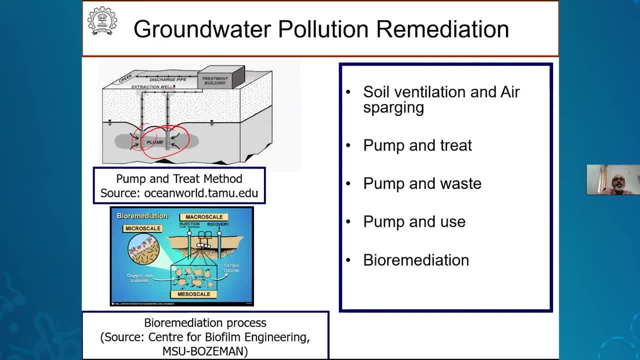 contaminated. what is uh is taken out through pumping well, extraction well, and then the treatment building is there and they're treated and then you can either put back to your cream or you can directly utilize it. so that is called, which is our on-site technique, and then uh, in situ bioremediation you can see here. so this is a bioremediation technique. so 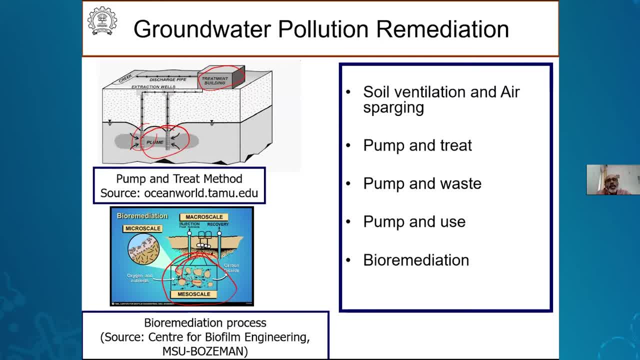 this area is polluted. so he identified the, the bacteria, and then you are allowing that bacteria to grow there by supplying oxygen and other nutrients and then, uh, that will be automatically will be treatment. it will take in place in the soil itself or the aquifer system itself. so, uh, um the like assignment: soil ventilation, air sparring, pumping, pump and waste. 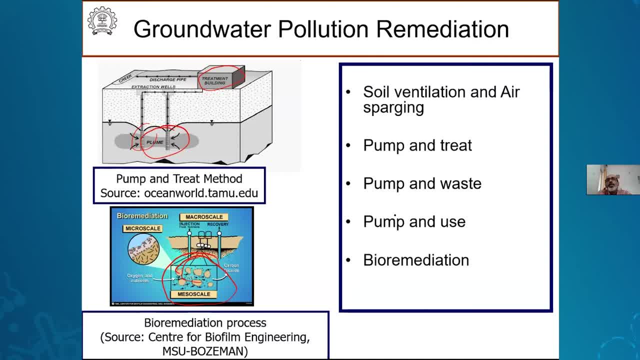 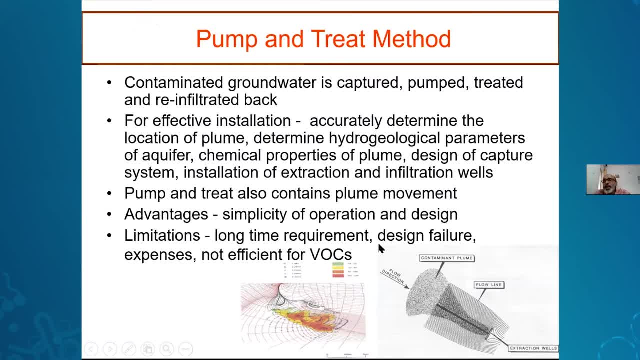 pump and you use so like that. these are some of the most important tools which we use for uh, for remediation. so, as i mentioned, pump and grape is very much used- though in india we have not experimented this, but uh in uh germany, spain and many countries, even when, while i was, 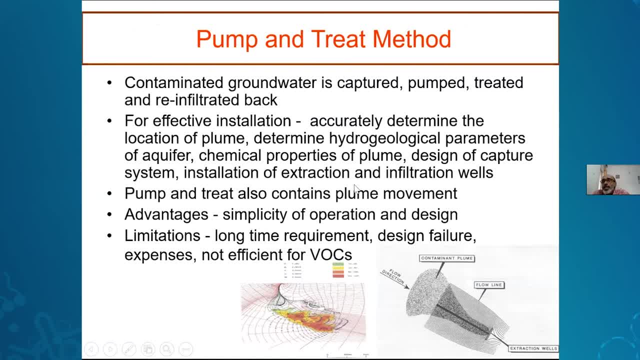 working in germany, i have seen many plants where there are especially municipal areas where people are using pump and treat and that is running. the plan is running for even so many years. so here, as you can see, here, what is this is, this is your um condemnation. so what we do, we can put. 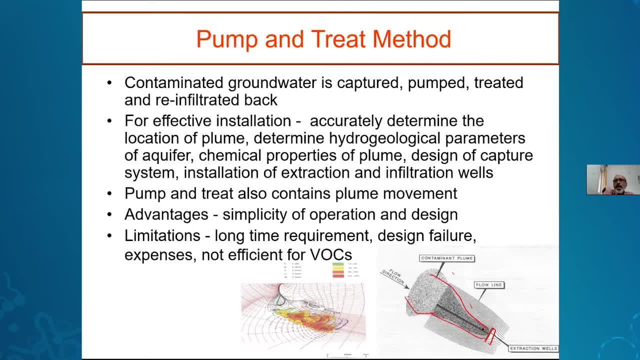 a series of wells here and then this room is captured and then contaminated water is pumped out. so condominium ground water is captured, pumped and treated and you can re-infiltrate back if it is needed. for effective installation accurately, we have to determine the location of proof, determine the hydrogeology parameters, except the pump, and it also can improve movement. 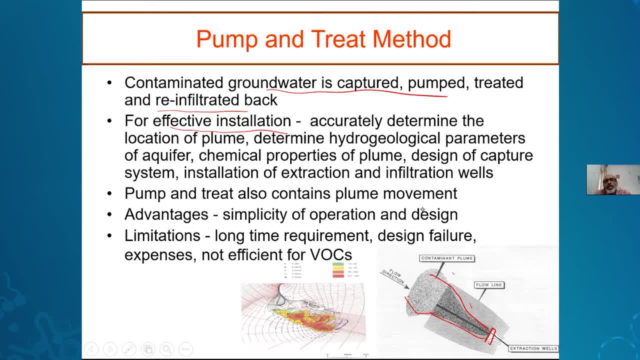 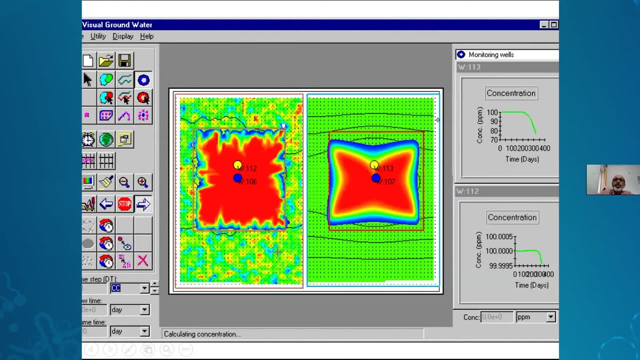 so the advantage is it is simple operation and design. but limitations that so many years are required, long-term requirement, design failures, expense. it is highly expensive and not efficient for volatile organic content. so this is what this. this animation shows what is happening in the pump pantry. so if it is homogeneous isopropyl media, it is easy. so you can see that this is a very fast we. 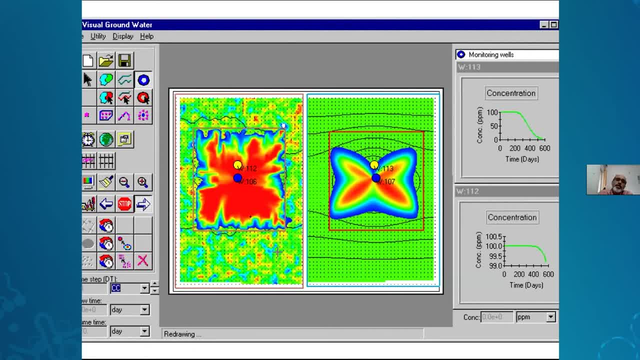 can capture the contamination, but uh soil is very much heterogeneous reality. is this bigger? so this is what you can see, the reality. so then many times we will not be able to even capture all the contamination. so that is what is the issue with, especially with the pump and treat. so then bioremediation, as i mentioned, it is a very 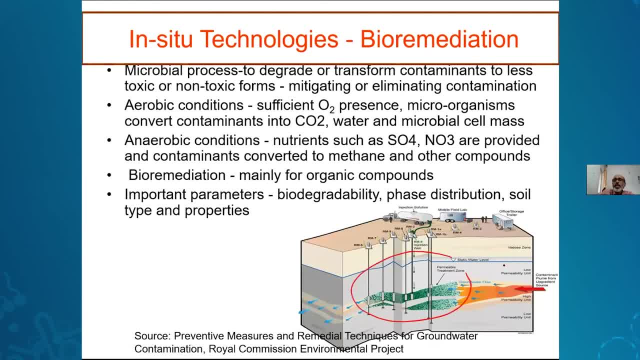 promising technology. so this is what we can see in the bioremediation. so here, if the contamination is flowing like this, so then we introduce nutrients and oxygen through wells and then that will be, uh say, here the bacteria quality will be enhanced, the microbial process to bigger. 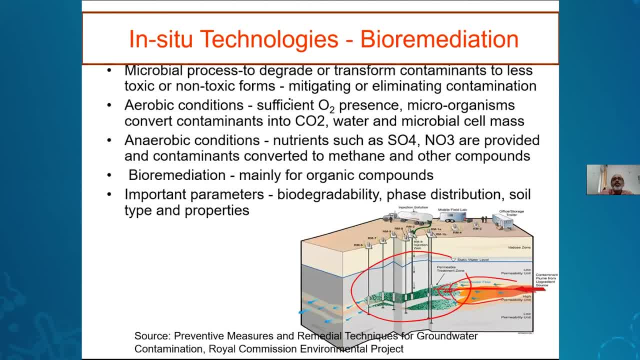 transform contaminants to leave toxic or non-toxic forms by mitigating or eliminating contamination. the aerobic conditions is generally, if you put oxygen presence means aerobic and and we can- that will convert to carbon dioxide. water and anaerobic conditions means and nutrients such as sulfate nitrate etc. also can enhance the the growth of the bacteria. 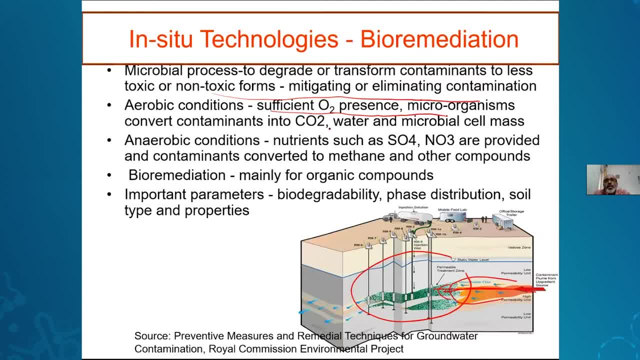 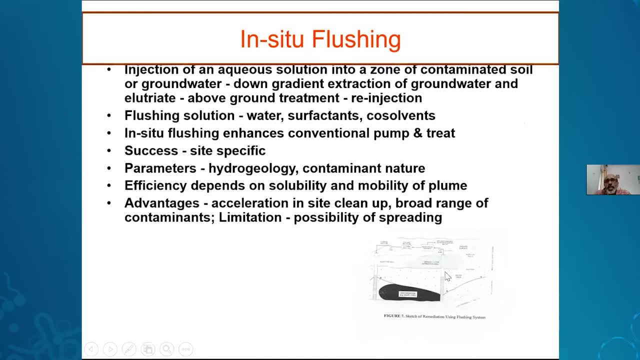 and bioremediation. mainly we do for organic compounds. so that is where you can see that the bacteria can destroy organic compounds. so this important parameter like biodegradability, phase distribution etc. should be known for this and then another technique which is used in some countries are called in-situ flushing. so for 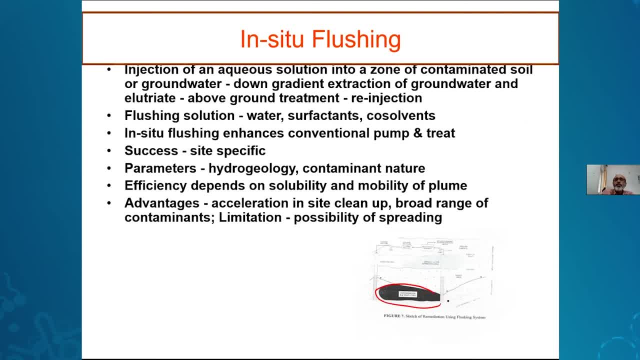 example, if you identify them- and i'm in clue, since this is really the moment of the plume is so slow, as you have seen, it can be many, many days or even many years. so we, whatever you do, we inject your solution to zone of contaminated soil or groundwater down gradient and flushing solution like water. 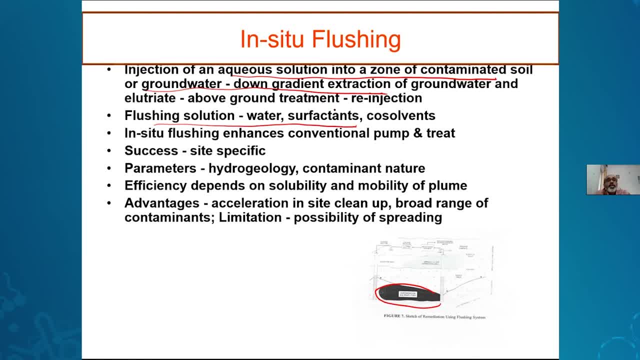 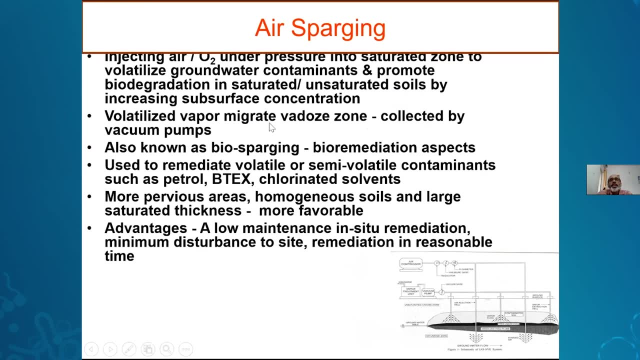 surfactants, cost solvent which is not polluting the groundwater. so in situ flushing, enhanced conventional pump pantry, and the success depends upon size, specific, so you need to see various parameters, and efficiency depends upon solidity and mobility of it. so that is called up in situ flushing and then you can see air sparging. so, as i mentioned, if it is a quality, organic, 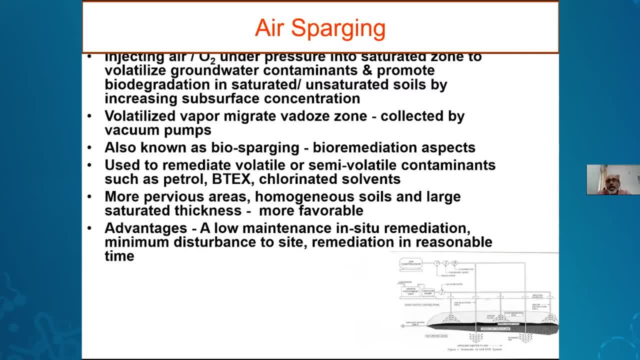 condominium center. we can inject oxygen or air in a high pressure and that can converge, like it detects uh. problem solvent this uh. it can convert into uh, say by putting air. that will be the contamination of the converter. so here advantage: low maintenance, in situ remediation, etc. 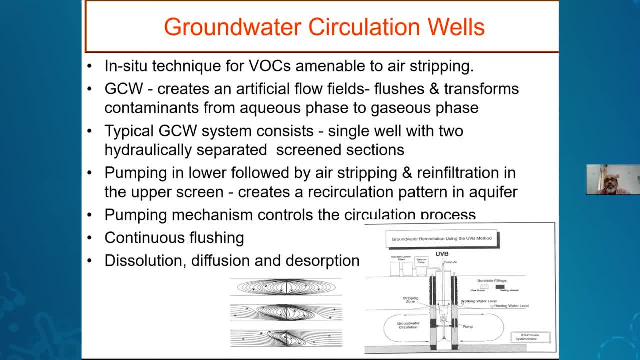 so these are the the advantages of uh airspan. so one important innovative technology developed in germany is called groundwater suppression, because actually i was also working in this area there while i was in germany. so here, uh water. organic condoms are unable to air stripping, so here this is a well. 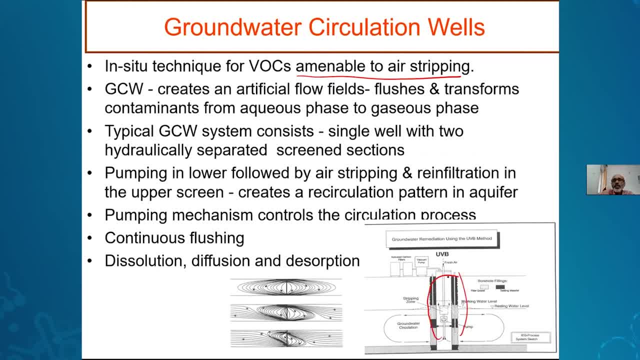 we introduce here. so there we. then we put: we supply air, and then uh- this is called a suppression zone- will be generated, and then it will be: air will be introduced. it creates an activation profile- pressure stands for contamination and uh from active space to the asia space and there's a 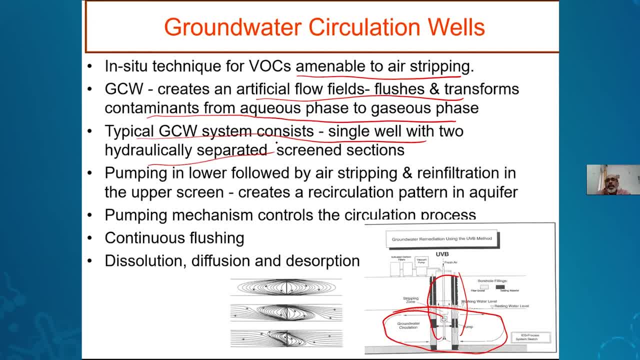 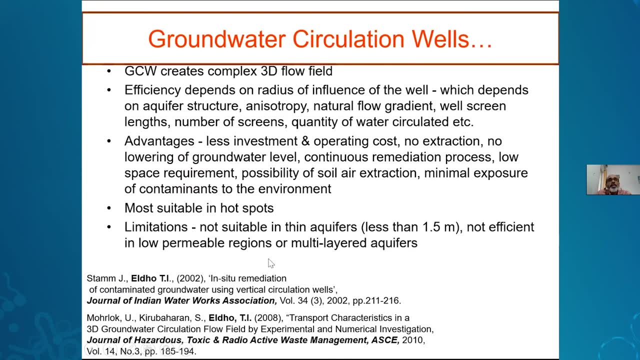 single well or multiple wells can be there, pumping in lower, followed by air stripping, re-infiltration at a space create a circulation zone, so this is called a circulation spot, you can see here. but the mechanics control the circulation process and then continuous flushing and dissolution, diffusion. all those things happens. so here, as you can see, it creates a complex 3d field efficiency. 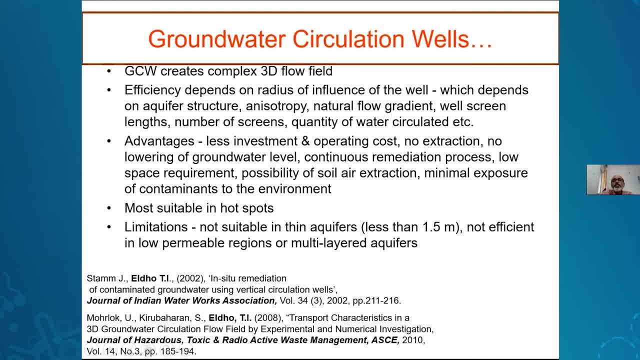 depends upon the areas of influence of the wealth advantage: less investment and there is no need to pump out the groundwater for water, but automatically base space. it will be uh, same, uh within that zone, or the, the, the, uh. the remediation will take place, but uh. this limitation is that we need to exactly. 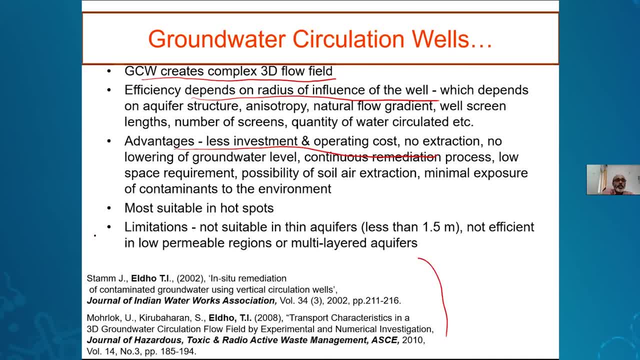 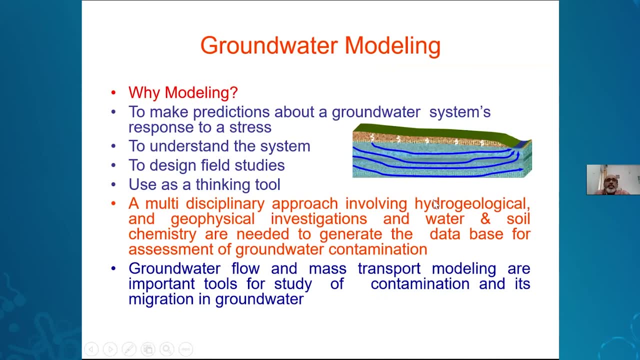 identify the location and those who are interested. we can see some of the papers which was published by me while working in this area. so then, uh, coming to now, another engineering aspect is so, as i mentioned it, so this system is so complex, so we need to model it. so that is very important, since 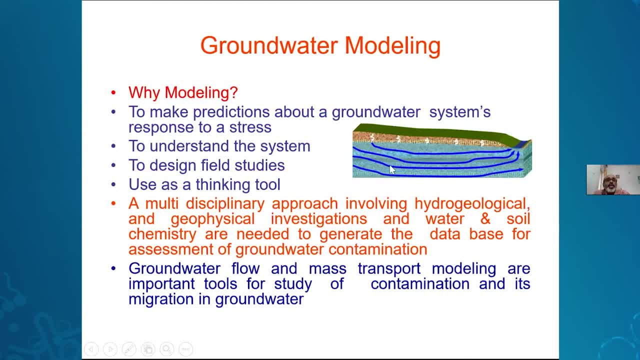 we do not know what is happening realistically. so that is why groundwater modeling is so important. so here, to make prediction about the groundwater system response, to stress: so, if we are pumping groundwater and how the groundwater will be behaving, uh, how the flow will be taking place, so we, to understand the system, we need to have a thinking tool, so that is called a model groundwater. 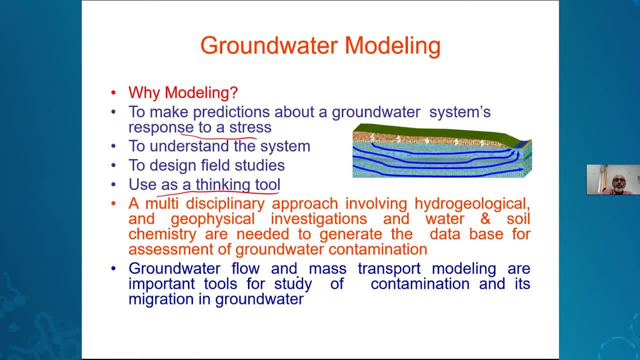 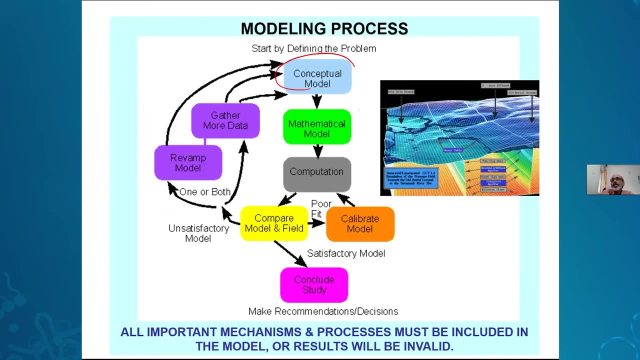 model. the multidisciplinary approach is required. so groundwater flow and mass transport are important tools for so we will have a transport model, flow model and transport model so you can see that we can conceptualize the area like we can be decided then. there are many equations like partial equation for flow and transport can. 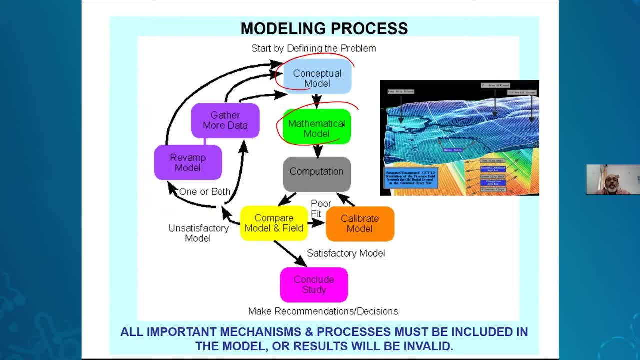 be obtained that is well developed in this area, and then we can solve those equations, computation, and then finally we can get there, we can calibrate and validate also, and then we can run the model and then we can get the- uh, various scenarios. so that is what is in the modeling process. 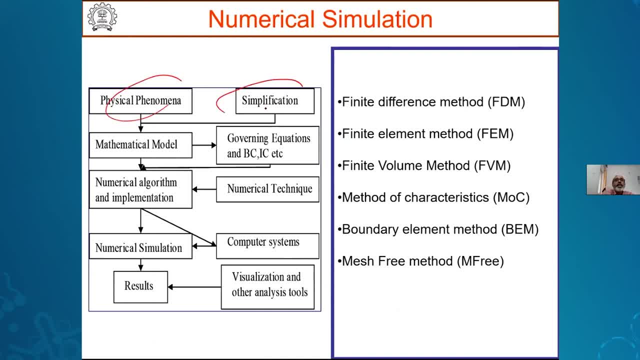 so here a physical phenomena, then we will be simplifying and then a mathematical model will be developed and then, uh, appropriate boundary conditions, initial condition etc will be applied and then, uh, we can have a numerical algorithm and implementation using numerical techniques, various techniques, like a final different method and method of finite volume, etc. uh, now, here days, we use mastery method. 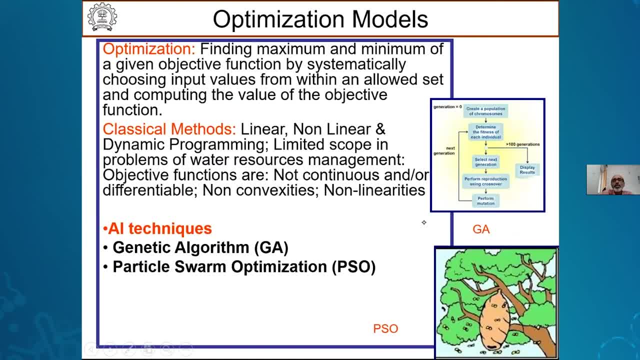 also so variety of methods. we can uh use it, so that is called simulation. so now, as i mentioned, if you are going for a remediation, then pump and treat or a biolumination- all those areas we need to optimize. also how much is to be pumped, how much you want. 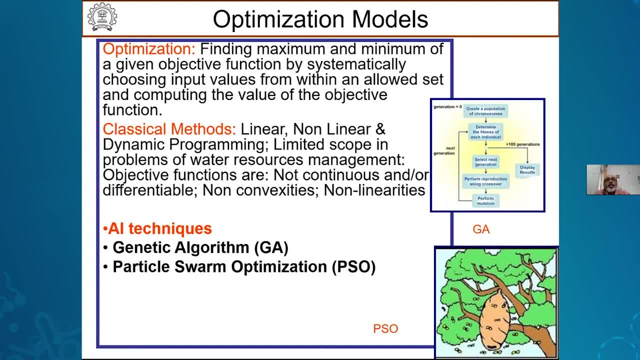 kind of control is to occur. so optimization models also. you can use it so to find the maximum or minimum given objective function, like with the minimized cost, maximum benefits. so it is what is will be always using. so for optimization, though there are so many classical methods nowadays, we 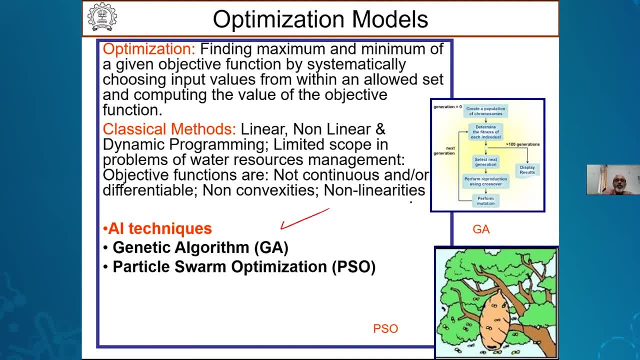 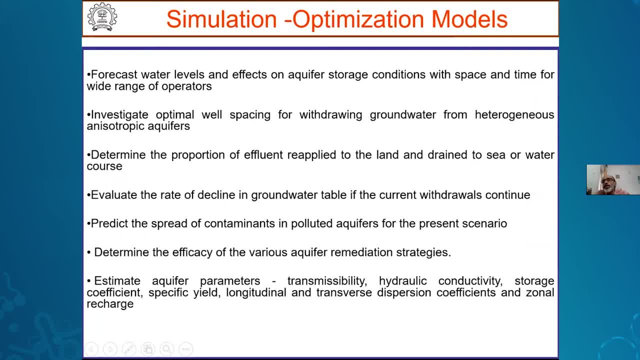 are using artificial engineering techniques like genetic or the particles of optimization, etc. uh, so simulation: now you can connect the simulation model with optimization models, so we have got a very powerful tool, since, as an engineer, since i am, a number of major students are working in this area with me and we have almost finished. 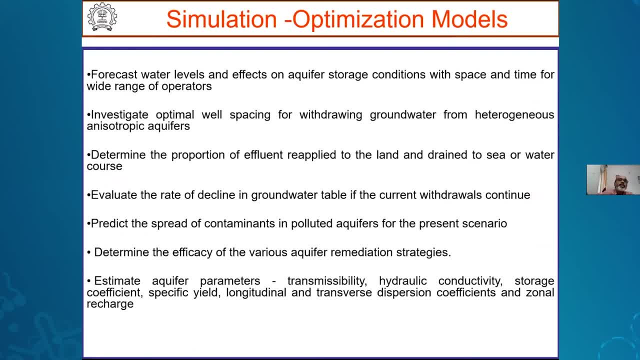 some 20 phds in this area. so here the simulation optimization model, forecast to water levels and effect on aquifer story condition and investigate optimal well spacing for withdrawing groundwater. then between professionally approved, reapply and evaluate the rate of decline in groundwater table. so, like that, various uh uses are there. so now, uh, that is uh. 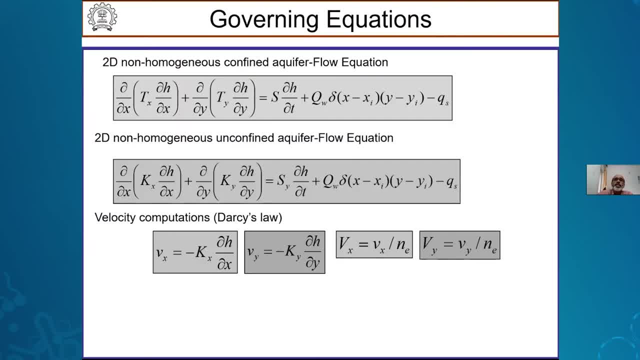 especially simulation optimization. so here these are the equations which we use for a groundwater flow, this is here for confined aquifer, this is for unconfined. so what we will do: h indicates the head, b indicates the transmissivity in confines. a keeper. k indicates the hydraulic conductivity, and 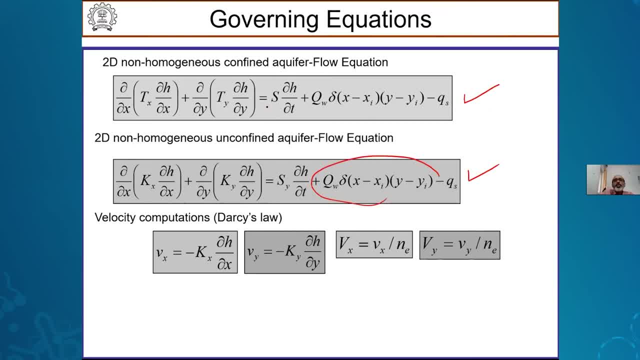 this is the public themes- uw. and there is this storey coefficient or specific storage. so that is a time-dependent equation. so you can see that this is nonlinear, partial difference. we need to solve this. by solving this equation, what we get? we get the head variation throughout. 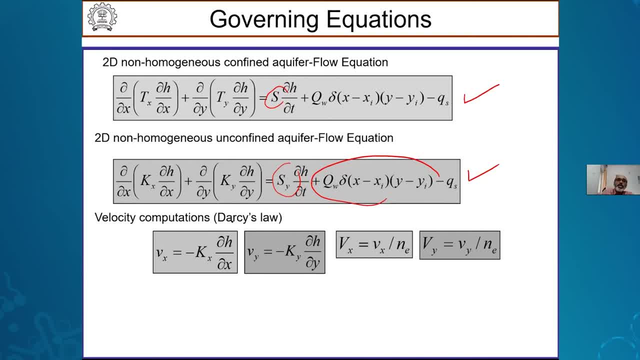 the aquifer system and then, using that head, we can calculate the velocities within the system and by darcy's law. so this is the, the velocity with respect to x, y direction, and then actual velocity can be calculated, and then that velocity- this velocity is value- will be putting. this is: 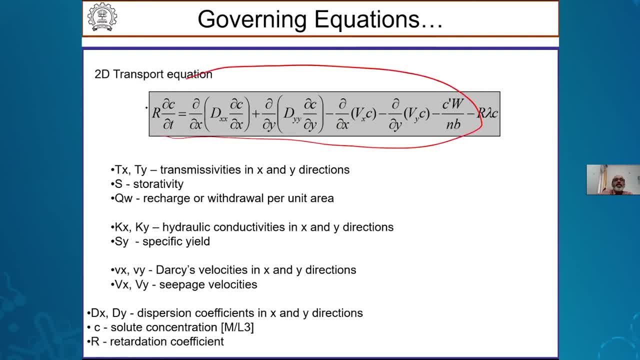 called transport equation, condamn transport. so here you can see, c is the concentration it can give us or any kind of whatever. you are putting so r into lc by delta. r is called a retardation coefficient, and then a dx is dy, y are called the dispersion coefficient, and here these velocities, 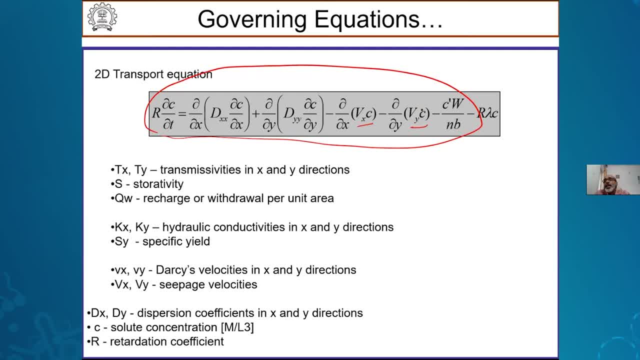 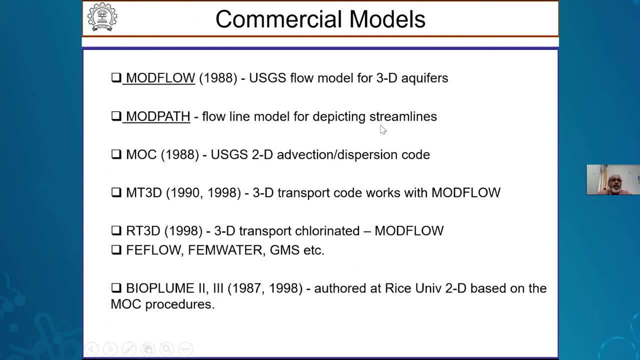 we need to get bx by, we need to get from the flow model which we have seen in the last slide. so then if there is a pumping or other kind of things happens, so that is the time. so this is called a 2d transport equation. so nowadays so many packages are available like mod pro, mod plug. 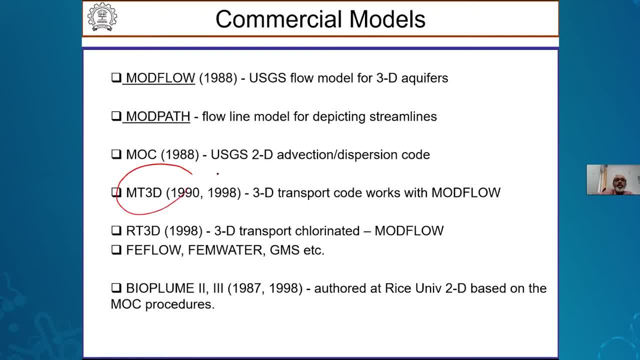 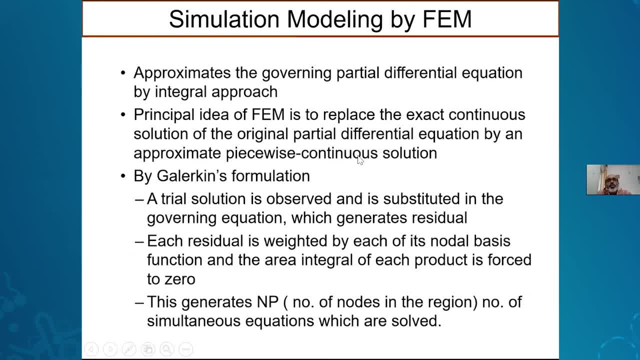 and then use it. so that is about the flow and transport model. so now, uh say, as i mentioned, filament method is very commonly used, so you see that even we have it in the common filter method. so here what we do, we replay the exact continuous solution by partial differentiation, by 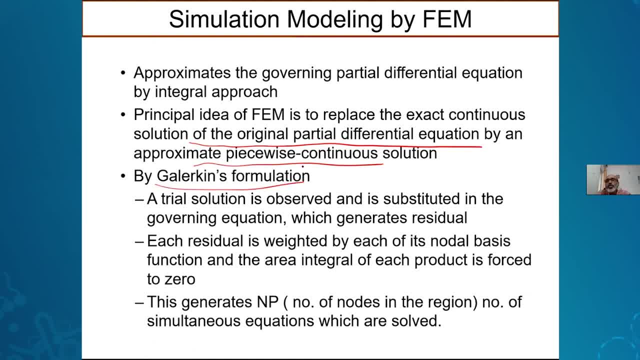 algebraic system equation the galerkin formulation is used. so those who are interested, of course our own lectures are available in the youtube and then you can look into that. so galerkin formulation is commonly used. so we converge this partially. first equation to an algebraic system. 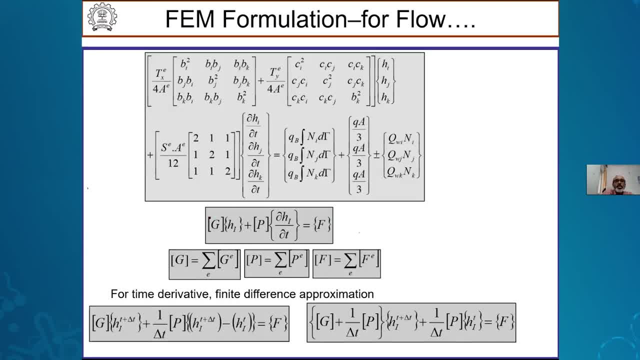 like this. so that is finally, a conversion is done, so this is called an algebraic system, and then we apply the boundary condition and then we can get the head variation or the concentration variation within the system. so this is for head, a flow, and this is for transport. 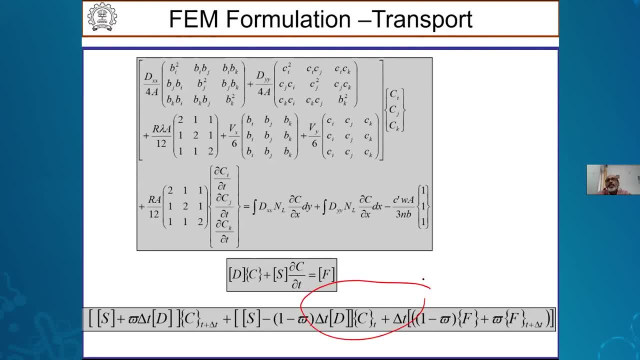 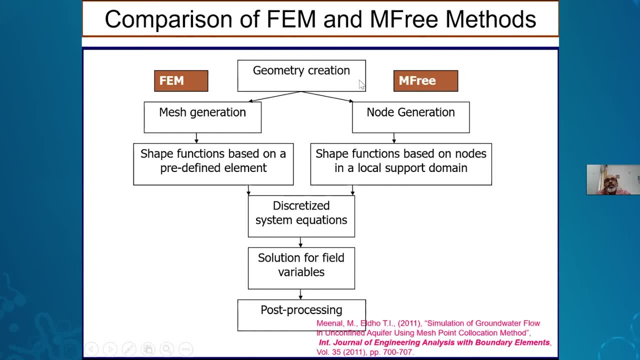 so finally an algebraic system is obtained and that there will be putting the boundary condition to solve the flow and transport. so here, as i mentioned, those are industrial simulations. so recently we have developed a mesh free method also, so their pattern method is concerned, we need to. 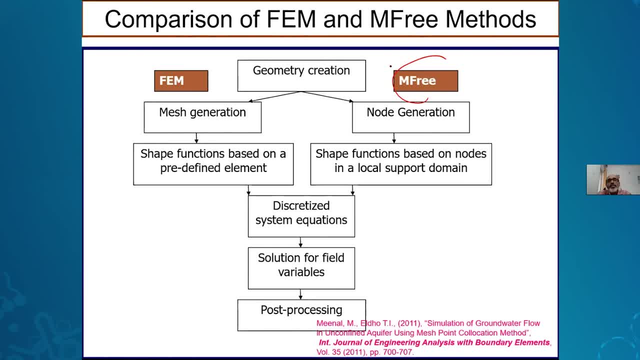 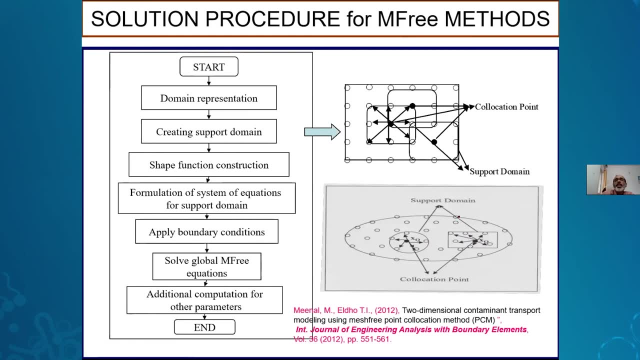 have meshes and that mesh is, development is difficult, so that is why mesh free method is developed. so there we simply, from three functions and those who are interested, some papers. we have published number of papers in this area, so you can see that this is mastery method. so we put only throughout the nodes, the domain, and then 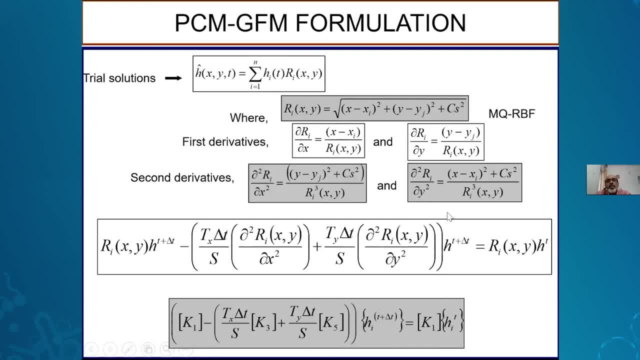 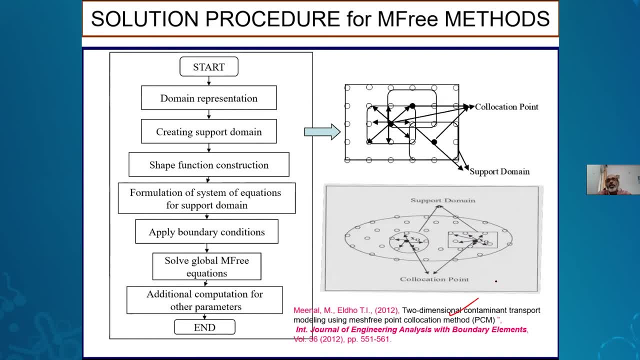 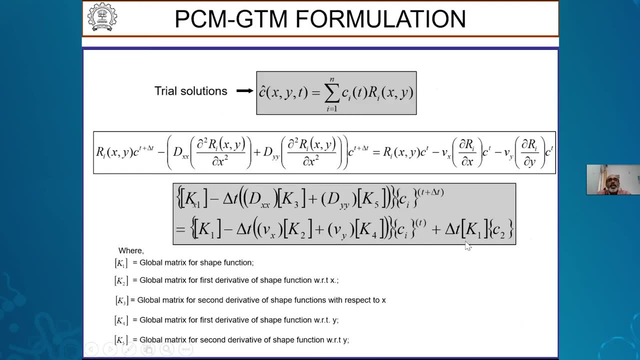 we can use this for simulation purpose, so that is so called a mastery method. i will not go into the mathematics of this. those who are interested. so papers, number of papers are listed here. those papers you can download. even if you search with my name, you can see these papers. so now finally, very 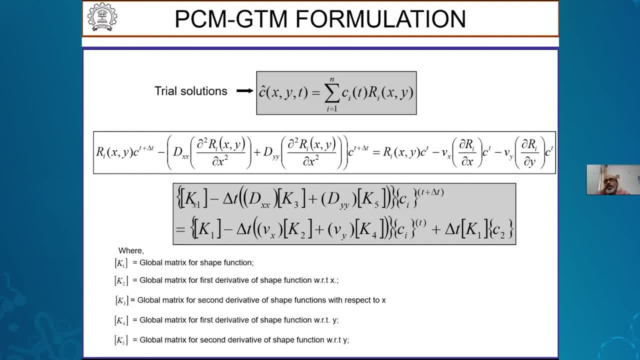 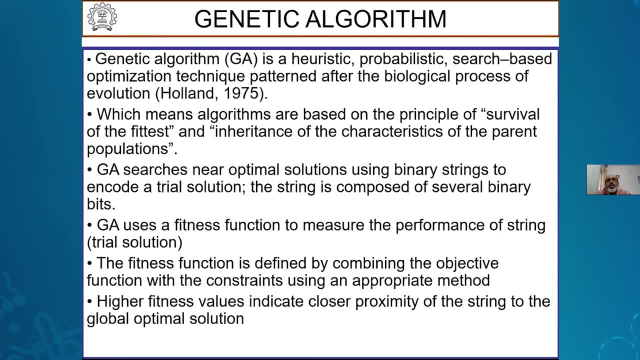 similar to some final time method. so now, finally, very similar to some final time method. so now, finally, very similar to some final time method, measuring method also. we convert the flow and transport equation into algebraic system and solve it. uh, so here then for optimization, we use the two techniques. one is called genetic algorithm, another. 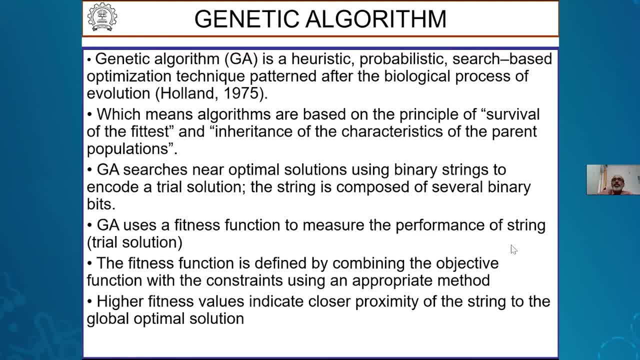 one is called particle sum optimization. so genetic algorithm is a heuristic, probabilistic method. so this is for optimization: optimize. we minimize the cost and maximize the benefits. so that way the genetic algorithm uses a fitness function to measure the performance of travel function. higher fitness values indicate closer proximity. so here, uh, first we encore model parameter. 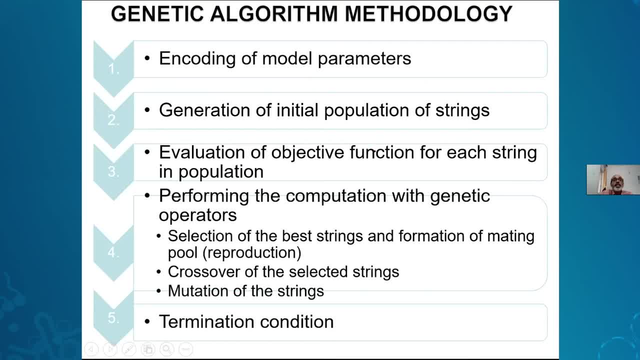 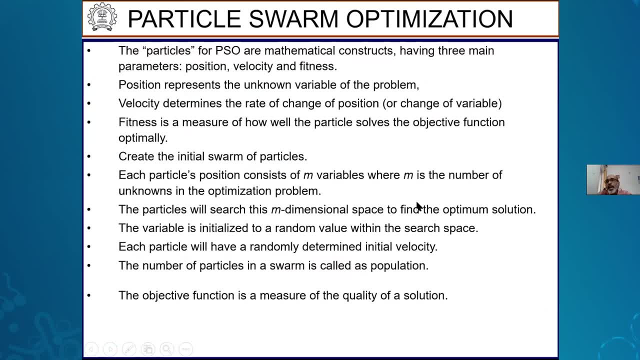 parameters and generate initial population and evaluate objective function and then perform computation and then that termination condition is applied. so that is the genetic algorithm. and another year recently, the recently used technique is called particle sum optimization, so they are like bats are flying, or then how? that pattern? based upon that pattern, we can create a swamp. 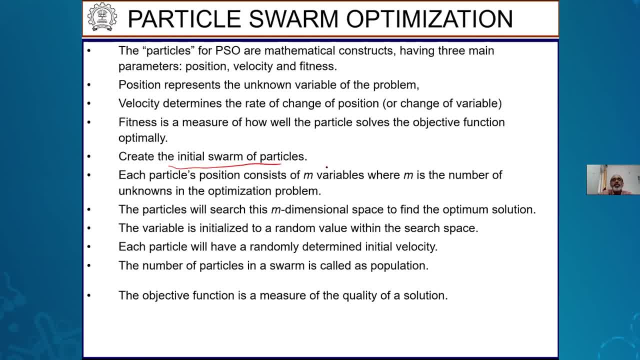 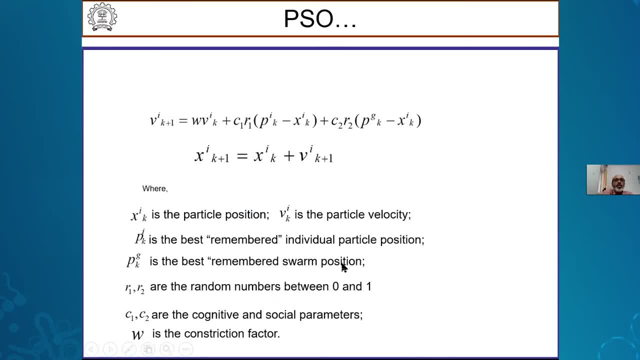 and create a sum of particles beneath the particle position consists of m variables varying the number of unknowns in the optimization and particle will reach search for this m-dimensional space and then we can get objective function measure to a quality of a solution. so here this is so called equation, which is uh, uh say the the. 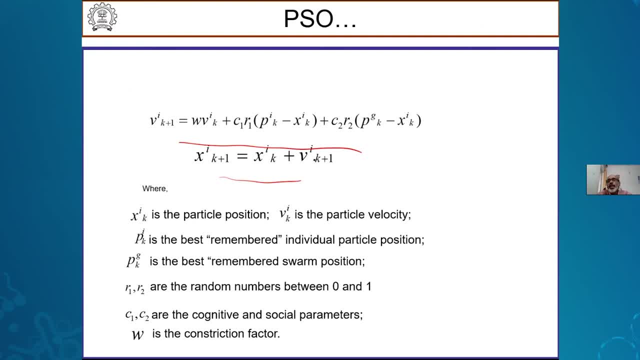 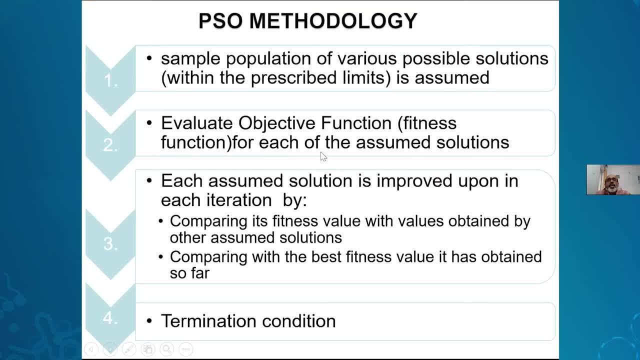 velocity or the movement of the particle and from that we can uh. so these are all generated through a random numbers and then using that, this equation, we can get it. so pso is again a sample population generated. variety, objective function: each are similar position, solution is improved. 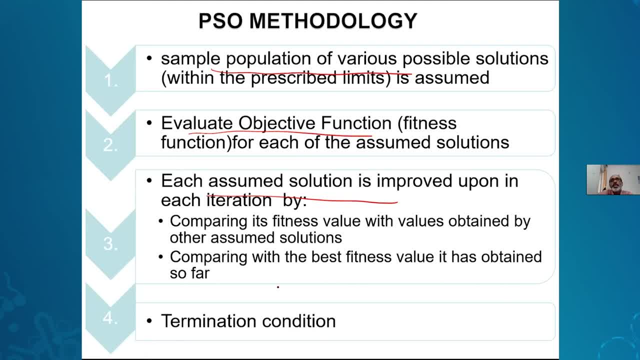 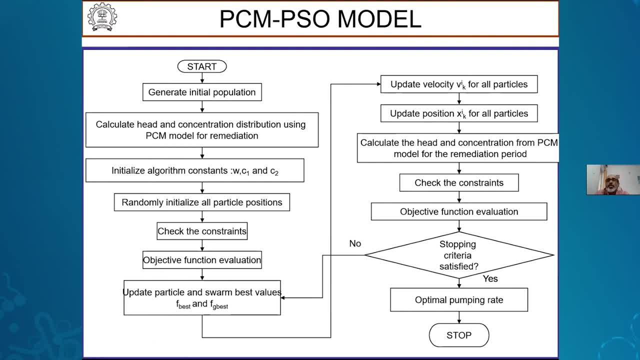 and comparing its weakness. finally, a termination condition is, uh, obtained. so, as i mentioned, what is the what why i mentioned this thing? so this is a lot of mathematics that you don't have to worry. we can develop a simulation model using finite element or measuring method, and we can 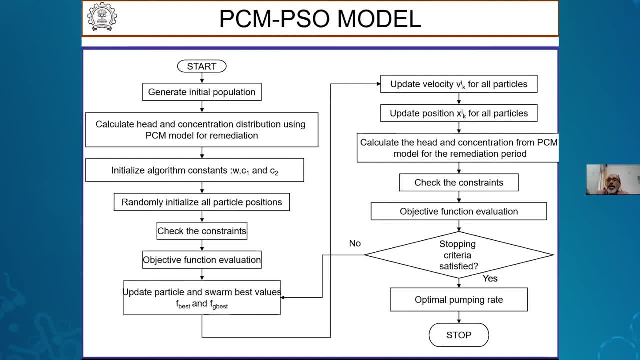 develop a optimization model. both can be combined together so that is called simulation, optimization model and that can be effectively used for is the groundwater, say, like a pump and treat or bioremediation. all this area we can use effectively. so this is a typical flowchart to is a part of the measuring method and the particles of optimization. so before 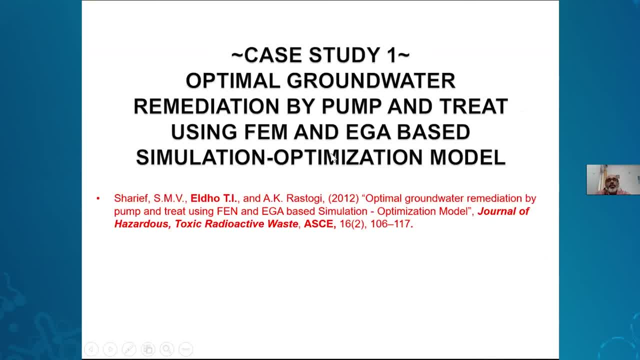 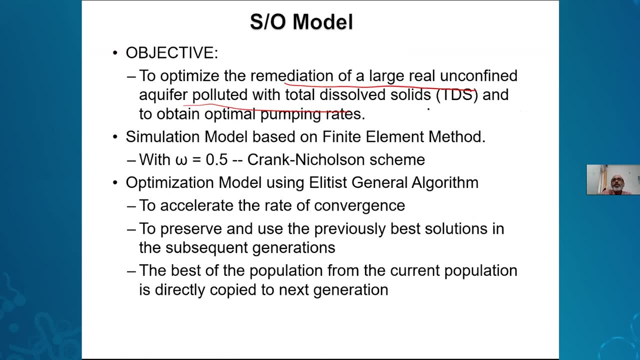 crossing. i will just briefly go through two case studies. one is on optimal groundwater remediation, like pump and treat, using a finite element and a elliptic theoretical simulation of industrial model. so here uh purpose is to optimize the remediation of a larger unconfined aquifer. for you with the total dissolved solids. 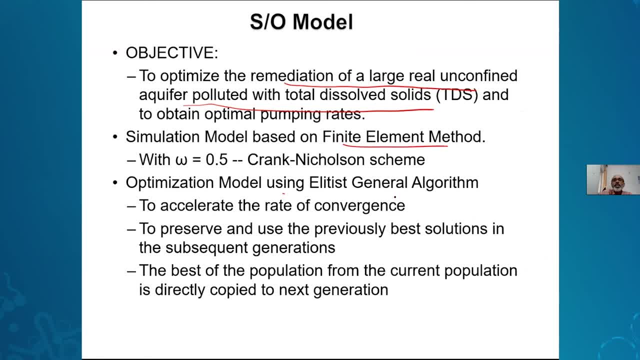 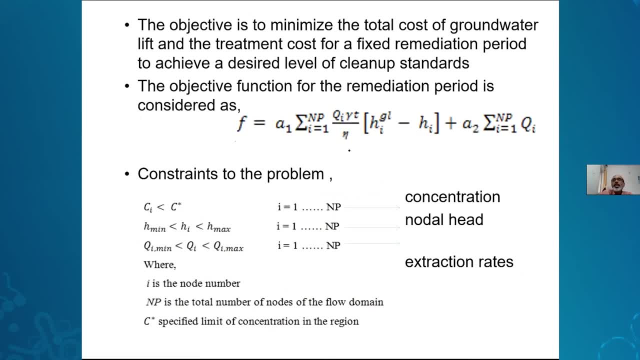 and the simulation model is the final method, and optimization is by genetic algorithm. so this, anyway, that may not be interesting to you. so here the objective function. so here we will be. in pumping method, we have seen that we need to pump a lot of water, and so that is one uh optimization. 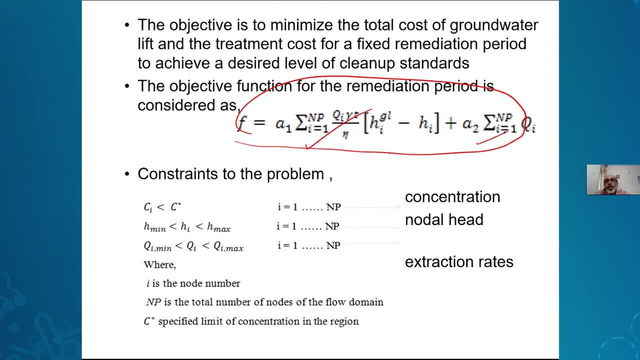 and another one is we need to treat that water. so that is, the total postage should be minimum and so that some of the constant- like okay, our dds, if it is 3000 we want to reduce to 500 or 750- head variation should be under the control and how much, uh, pumping should be taking place. so 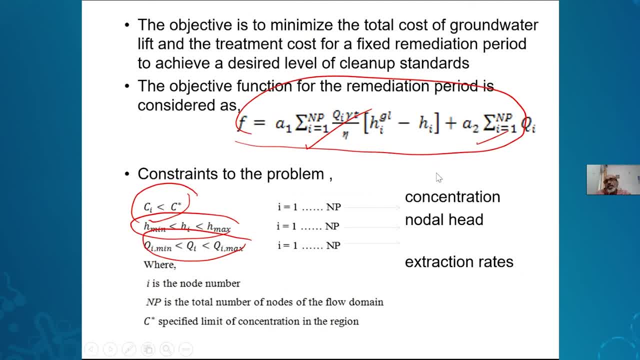 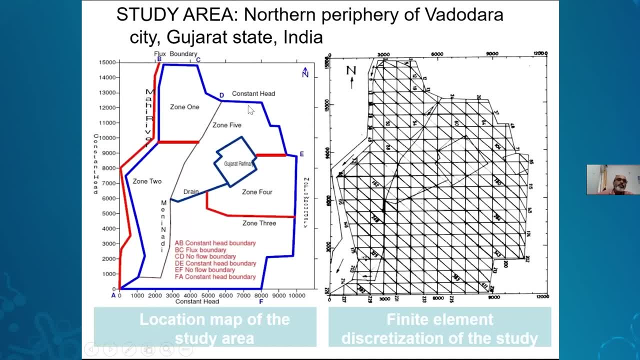 that is the optimization. so this model, one of my ph is to develop and apply for a, an aquifer system. this is in gujarat, only baroda or vadodara, so mahi river. so this is the gujarati refinery, this area. a lot of pollution in 1970s and 80s took place and then a prune was identified. 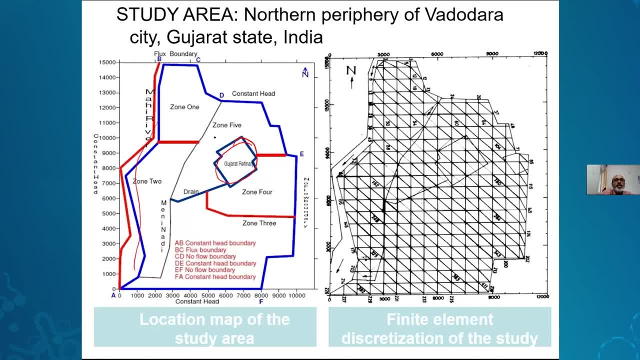 here, and this is a river, is mahi, though, is flowing like this, and then there is a small system is also there. so the aquifer system is various ones are shown here, and we use the final tournament grid like this, and then you see that these are the proofs. so this is one matter from. 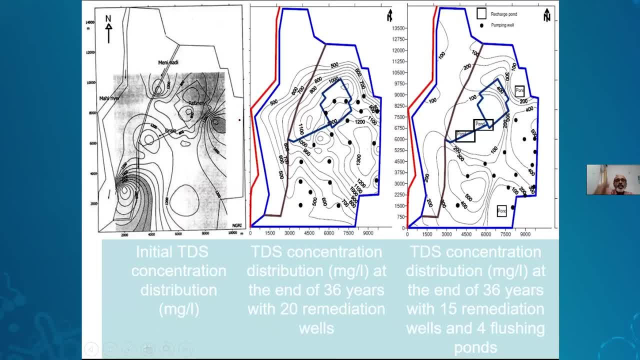 another problem like that. these are the proof which you can see here and here: tds concentration. each is about. you can see that it is about um, up to 2000, some hotspot, and then we need to- uh, we use the simulation optimization based on time turn and method and genetic algorithm. 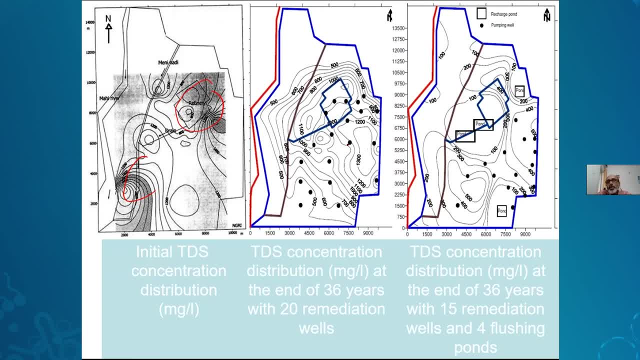 and the tds concentration we want to reduce to 750 ppm and that is what it. so, this being a large area, so area is about 150 square kilometer area. so it our model shown that we need to put 36 years of combined rate of 15 remediation wells and also some flushing, also required flushing bonds. 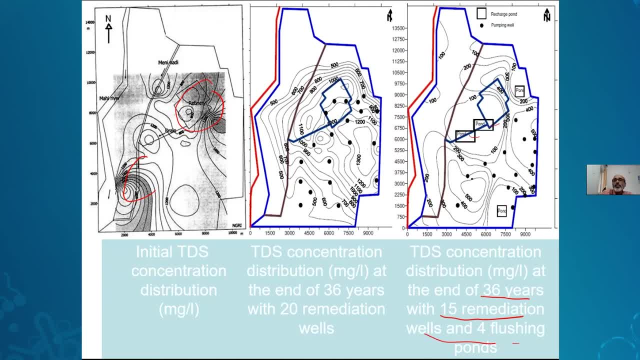 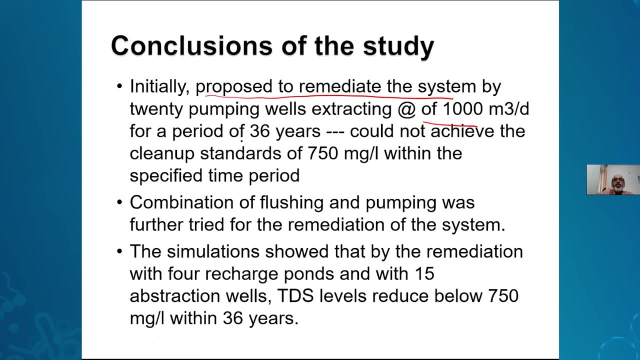 so this is the flushing bonds location, like four points are supposed, so that contamination from 2500 to we can reduce to around 750 ppm. so you see that here it is so expensive. the conversion is proposed to remediate the system and we need to put so much of waters. 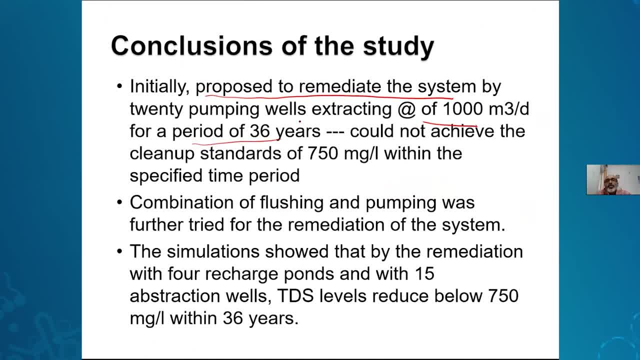 to be pumped out like a thousand meter group per day and to get into a level of 750 ppm and the combination of flushing and pumping is required and you see that um 36 years it may take. so you can see why it is so important to stop the pollution and the cost is here, about 66. 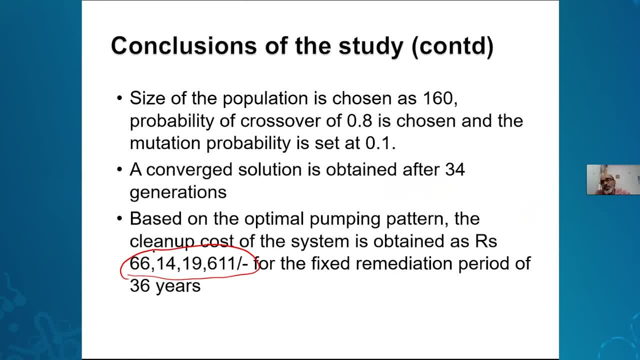 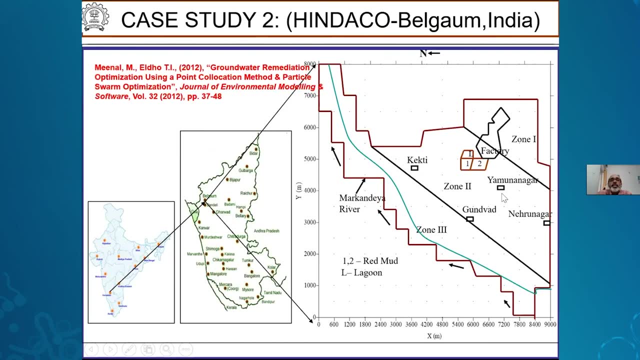 force rupees is required to to remediate this aquifer system. so why i put it in front of you that we need to be very, very careful, and then also we need to stop the pollution and how we can control the pollution. and then another case studies is in belgium. this is the industries. 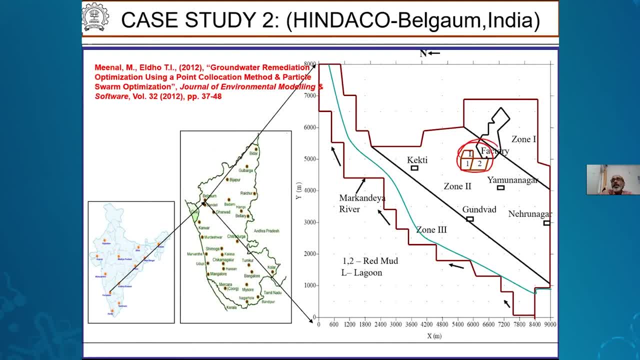 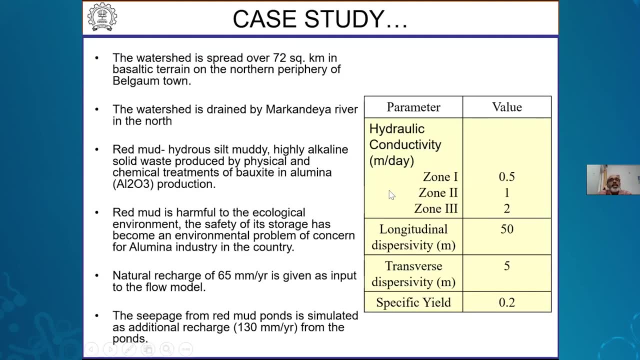 hindako. so here what they did is they have put some landfill with the alumina industries there. so there they put it like this, and from here a room was identified and this is an aquifer system. this is markandai river, and we did the simulation optimization model using mesh field technique here. 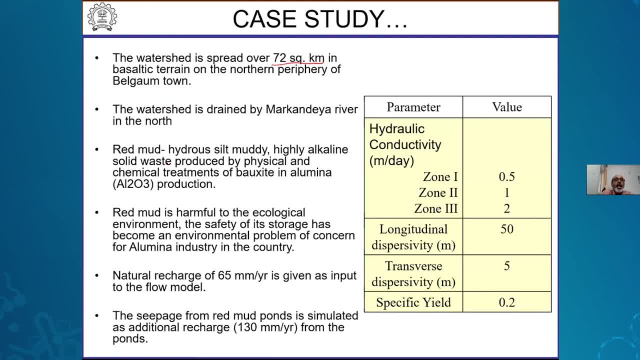 so here the area is about 70 square kilometer and red mud hydrols highly accurate. so this is from that. the tbs as a pollution and natural recharge is there, and then various things are put here. so this is the plume which we are adding the fact it is going up to. 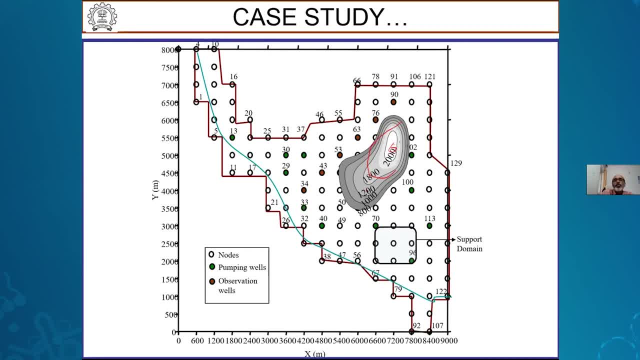 around two thousand at the hot spot and this is the the plume which we have identified. this is actually some report by ngri, so based upon that only we identified with this plume and now we used a simulation model. so for measuring models, so we used this many nodes and then simulated it, so you can see that how the groundwater variation. 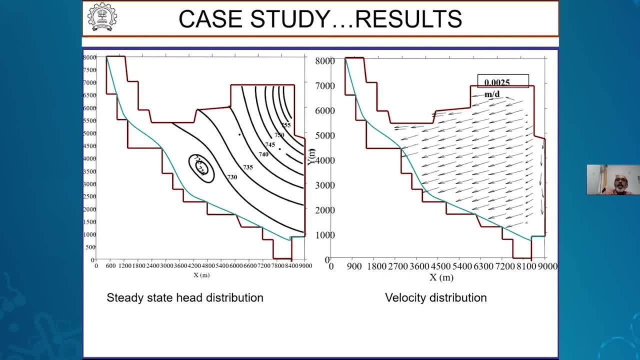 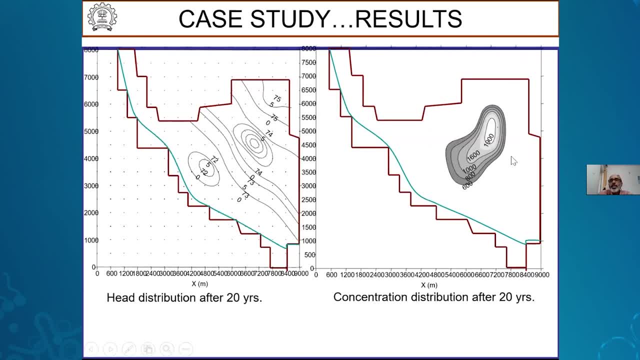 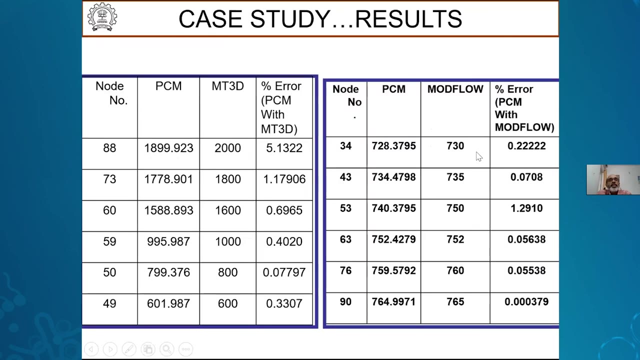 in this area. so here maximum and to minimum what is going this direction? so this shows the groundwater direction. and then our aim was so here and say after 20 years- since this is around 1995 or something- this contamination after 20 years, we simulated how it, how much area is this spreader using the simulation model and we compared with other. 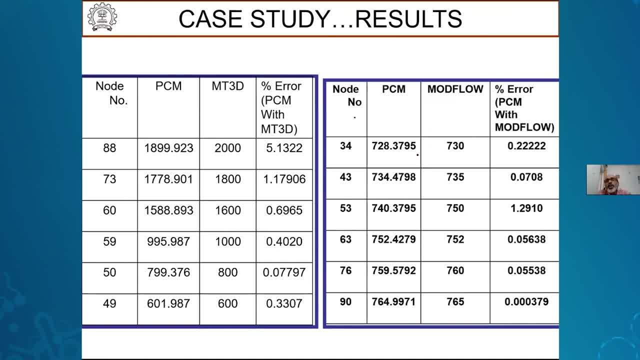 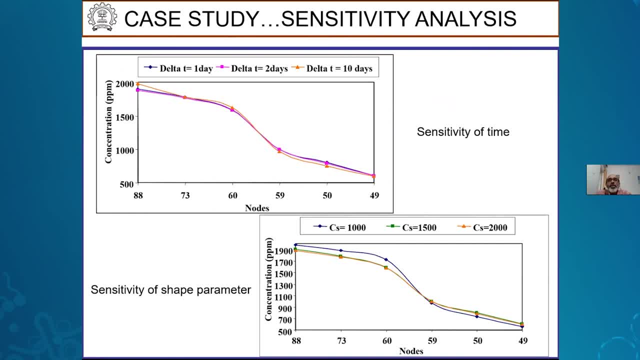 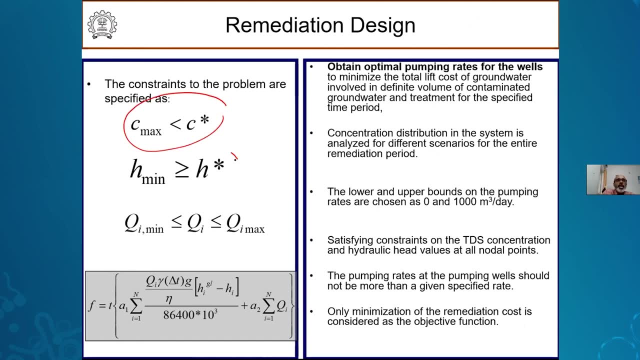 available models and then for flow and transport we developed the model and it was identified that we are getting very good match. and then we went for a simulation optimization model. so we used a particle sum optimization. so here this is our concentration and this is the. so this is the pumping cost and this is the the treatment cost. so that is a way, this remediation- 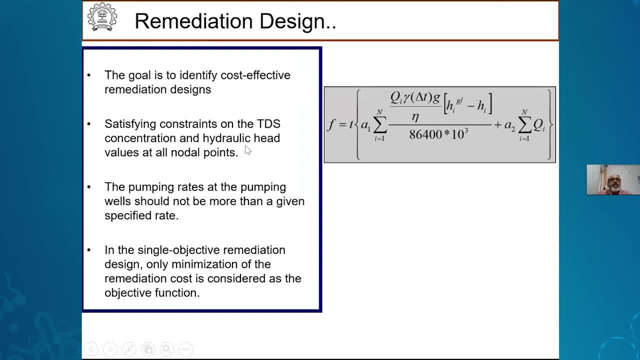 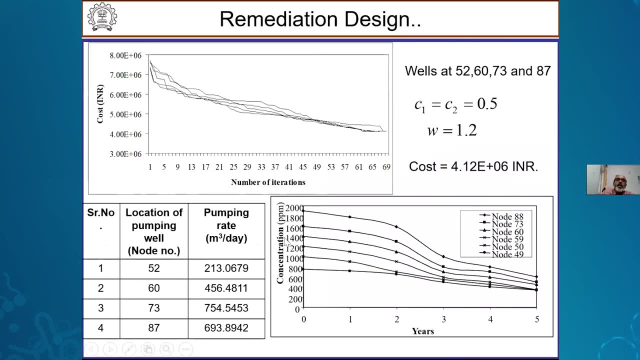 design is done and then you can see that the goal is to identify cost effective remediation design satisfying the constraints on pds. so this paper was published in the environment modern system by my phd students, so details you can download. so here: cost versus number of iterations and then 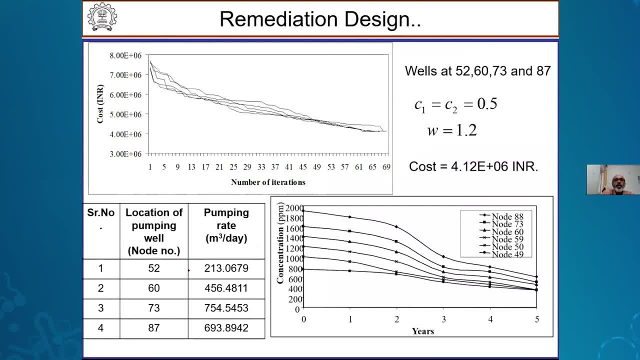 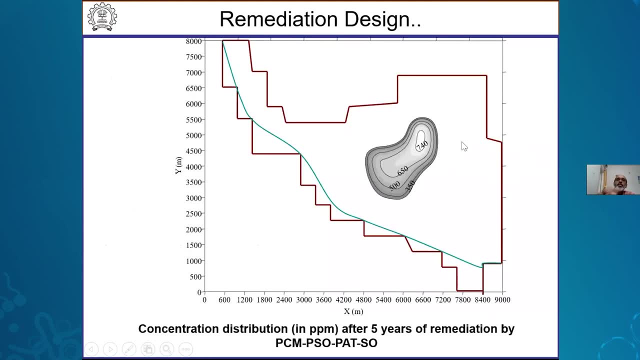 you can see that pumping rate, say four wells we proposed, and the cost is around, say, 41.2 lakhs. so that was the cost for remediation of this system. so here, once the remediation is done through the mathematically, it was shown that 750 ppm. this is the. we can get it using the similar. 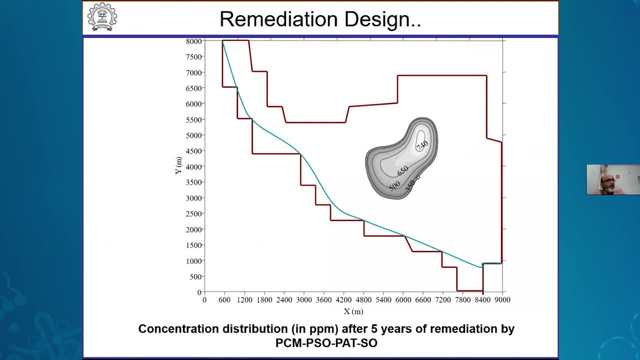 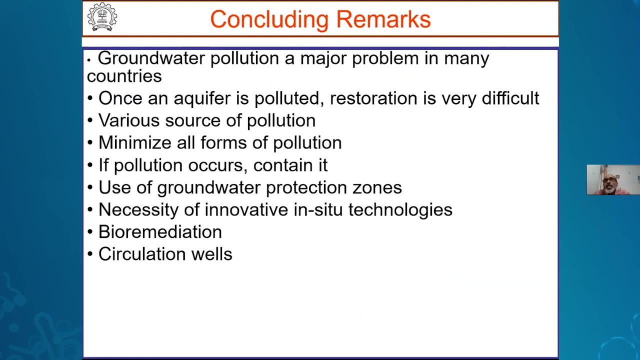 simulation optimization model, we can identify where is the, the source. so this is actually five years of remediation is done for this particular area, which we did using mathematical and simulation optimization model. so finally, to conclude, so groundwater pollution is a major problem in many parts of many countries, so especially in india. we are not so much bothered. 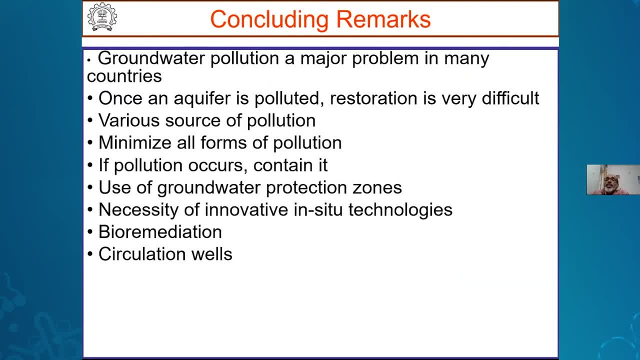 but now it is high time to look into this, since, uh, you see that earlier say, we thought in 1970s, 80s, the water is a pure source of water. that is what we thought. but now, due to heavy industrialization, agriculture, farming, all those, the ground is polluted. so once an aquifer is polluted, 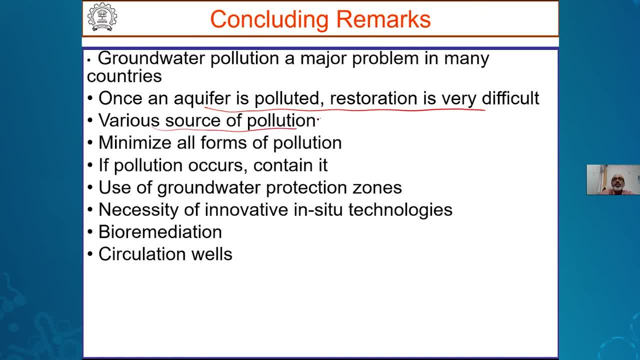 restoration is very difficult. so we have seen various source of pollution and then also our aim is to minimize the different forms of pollution. the evolution occurs. if pollution is identified, then a better thing is contained, so we should not allow it to further to spread. and then, as i mentioned, if you are using this groundwater for bringing another purposes, we 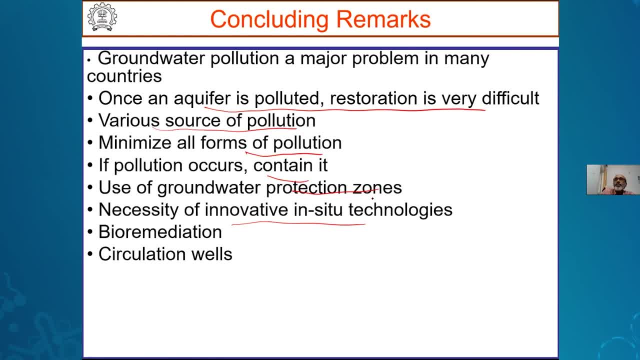 need to go for protection source and then, being engineers, especially civil or chemical or other environment engineers, we need to go for innovative techniques. so bioremediation as a country, since we we cannot spend so much money. so we have seen 66 crores or uh 16 lags. that depends upon the 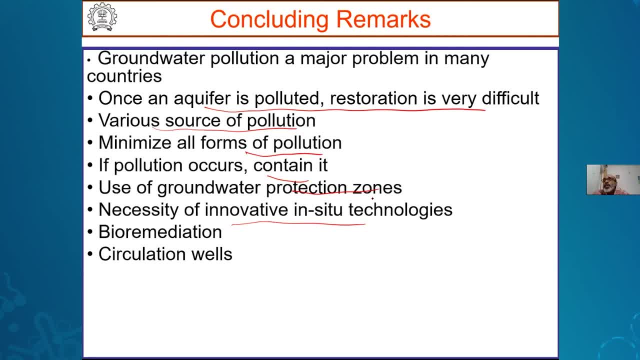 pool size, what kind of contamination, how much area spreaded- so all these things are a big question. so bioremediation is a very promising technique. so that is a lot of research work is needed. we need to identify the, the bacteria for each type of contamination and how we can enhance its. 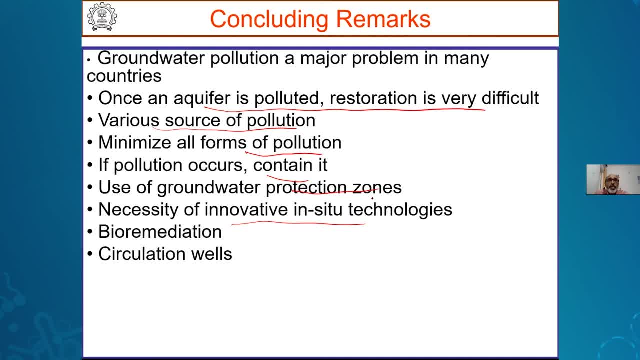 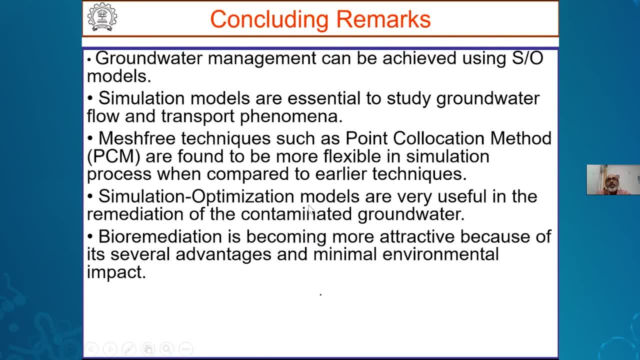 activities and then we can, how we can do the remediation. so that is we need to see and then like a circulation based, like in situ technique. that is also promising. okay, so groundwater management can be, as i mentioned, that through mathematical models, simulation, optimization model, we can do groundwater management. 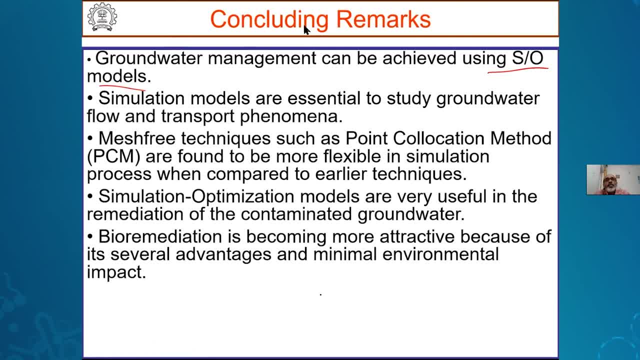 simulation models are essential to study groundwater, since the groundwater is very difficult to manage. so that way, simulation, modeling methods, or the final method, we can use it. simulation optimization, one very useful for remediation of the condemnation groundwater and bioremediation is becoming more attractive because it is several advantages and minimal. 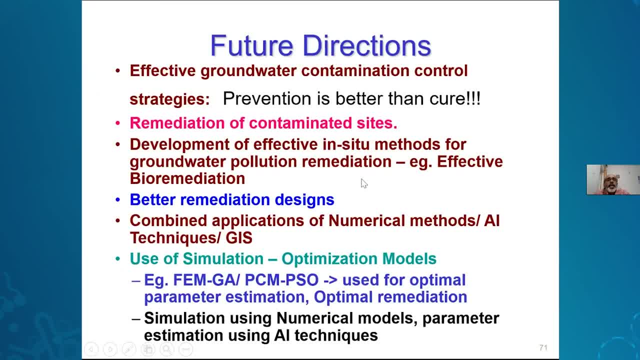 environmentally so. finally- this is the last slide- the future direction affecting groundwater contamination control strategies. prevention is better than cure, so we need to look into that way. so remediation of condom site is essential. development effectively in situ method, methods for groundwater pollution, like effective bioremediation. that is one of the best. 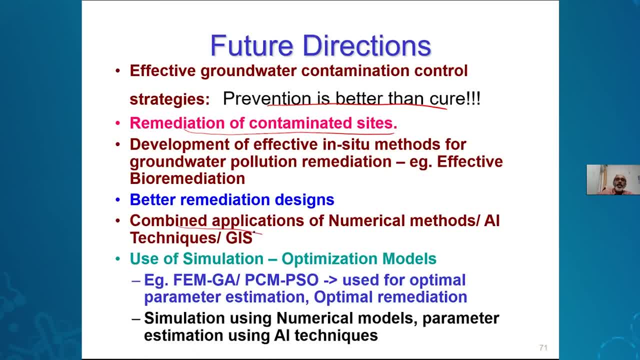 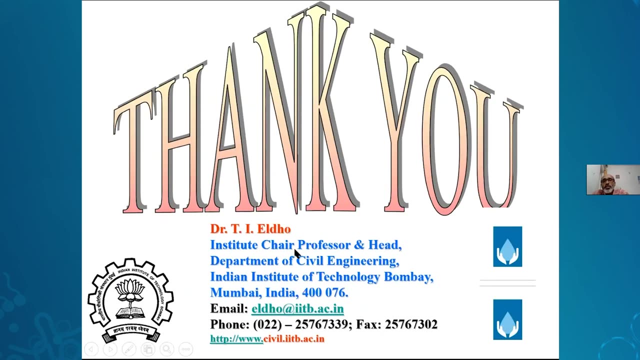 methods and then better remediation design we need to look into so like we can use numerical simulations or artificial intelligence tools for these kinds of studies. so further finite element or mesh method or general uh, then the artificial intelligence techniques can be effectively utilized. you know what remediation or designs. so that is about what i want to say today. so i have taken